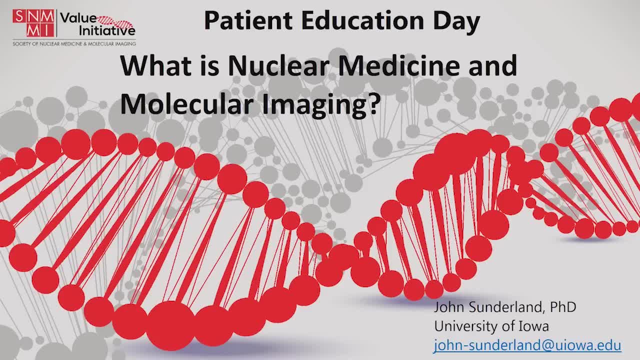 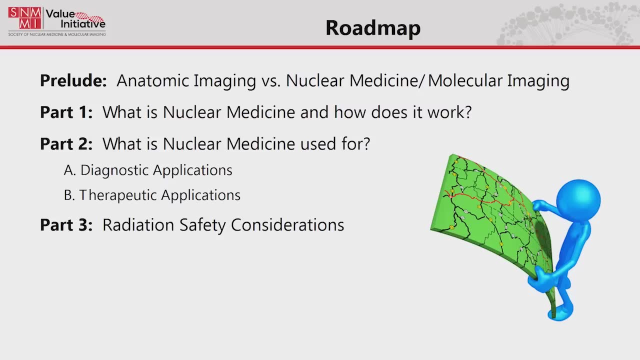 education, patient advocacy. So this is an important part of what the society does. So my charge is actually just to do a very basic overview of nuclear medicine, molecular imaging kind of how it works and what it does. I've broken it up into four parts. Just one slide on the difference between anatomical imaging and 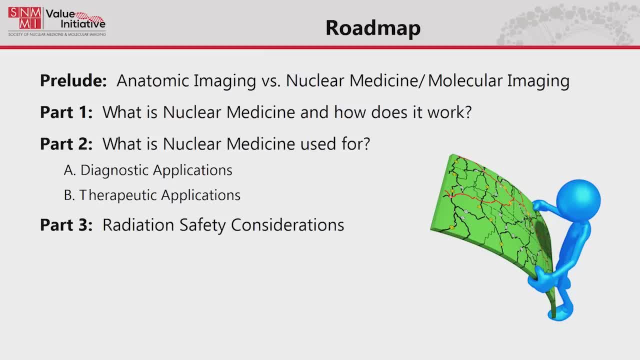 molecular and nuclear medicine, just to try and differentiate between the two, And then I'm going to demonstrate that from the get-go And then we'll talk about 15 minutes on what nuclear medicine is and how it works, kind of from a technical standpoint. Forgive me, I'm a physicist by training and so I have to do a little. 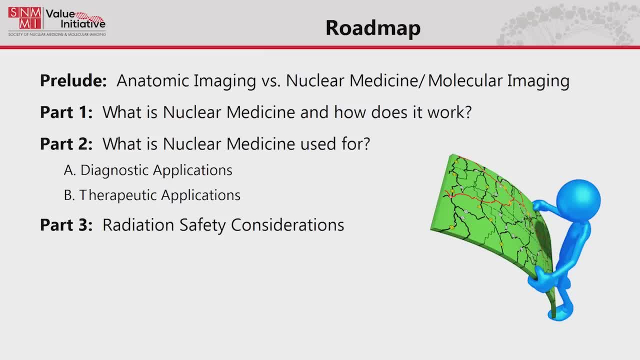 bit of that on the front end. And then, what is it used for? We use it for diagnostics, and we're using it more and more in the therapeutic arena, And so we'll get into that Both what's approved by FDA and what's coming down. 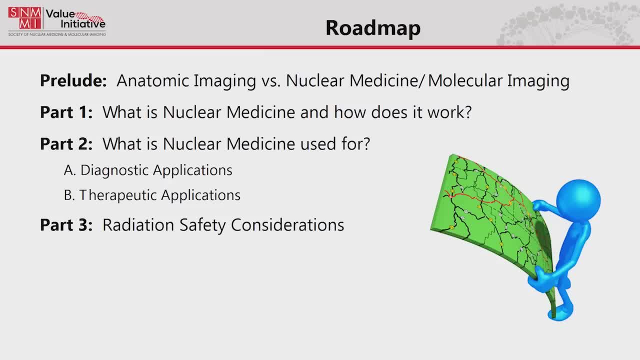 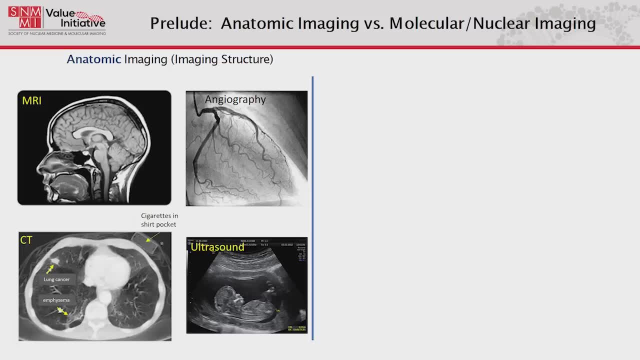 the road. And then a little bit on radiation safety considerations, as we are In fact dealing with radiation. So, just starting on the front end here, what you see in the upper left-hand corner, well, on the left-hand side, are some anatomical imaging techniques You're familiar, probably with most. 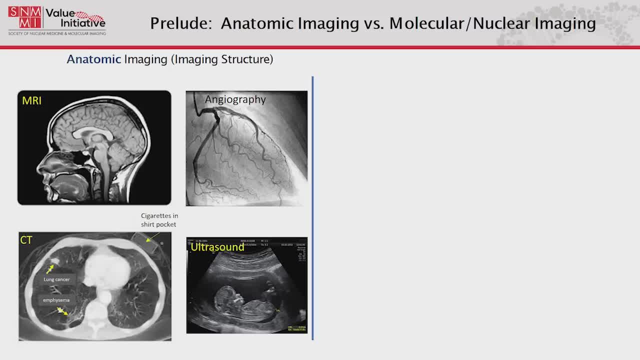 of them MRI in the top left. that's functionally imaging hydrogen or water density. It gives you great soft tissue contrast, beautiful anatomic images. There's a great diagnostic CT down there which shows a nodule which you can't really tell whether it's cancer or not. but you can see that little dot down there, You can see. 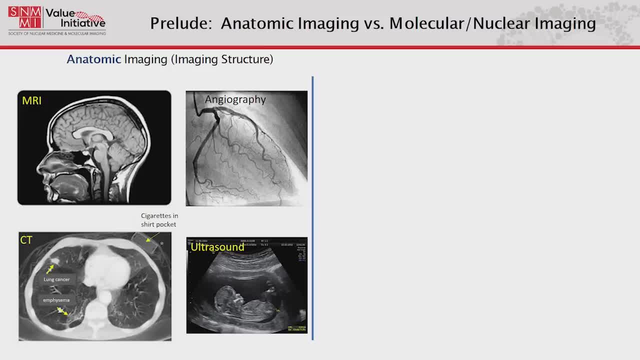 because of the pattern emphysema. And what makes this particularly diagnostic is in the upper right-hand corner, is the cigarette pack that's sitting there which helps the cancer diagnosis Angiography. by injecting dye in the veins You can actually in the artery of the vein. it goes to the arteries. You can actually look at the arterial blood supply of the. 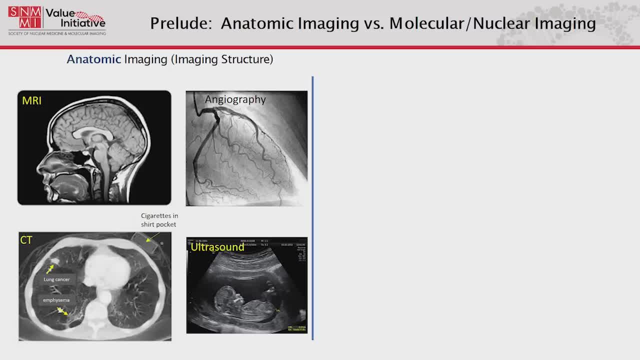 heart You can look for because of anatomy. you can look for stenosis and blockages there. Ultrasound isn't just used for obstetrics, It's used in cardiology, It's used in oncology And all of these are great and they have. 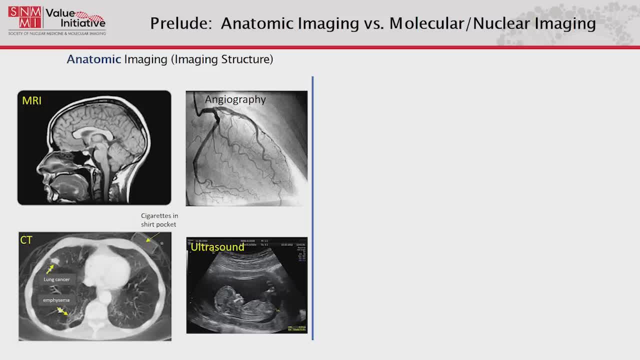 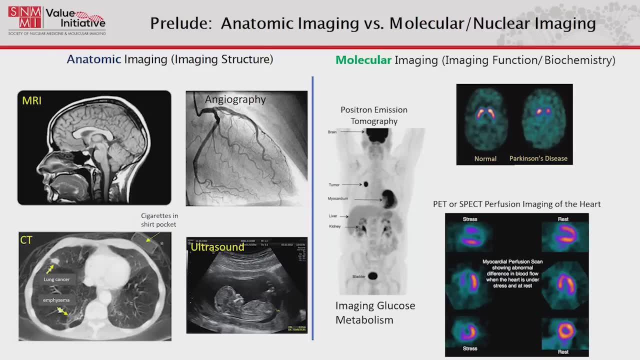 their uses. but they're all fundamentally looking at anatomy, Whereas in the molecular imaging, nuclear imaging biz we're largely looking at the biochemistry of the body. The anatomy is largely incidental. What you see on the left of that slide is one of our FDG scans. 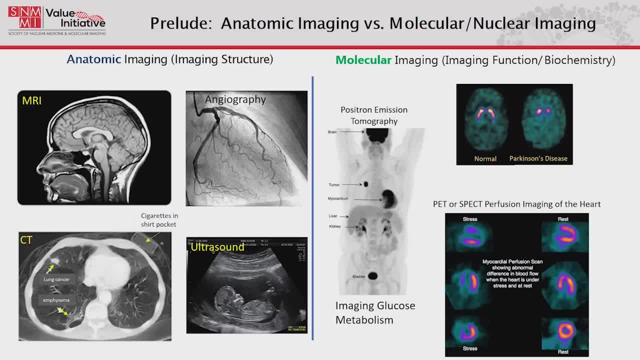 fluorodeoxyglucanase. And here what we're doing is we're imaging glucose metabolism. Because there's glucose metabolism all over the body, you can kind of see the anatomy, but that's secondary to the fact that we're imaging glucose metabolism. You can see the uptake in the brain because we're 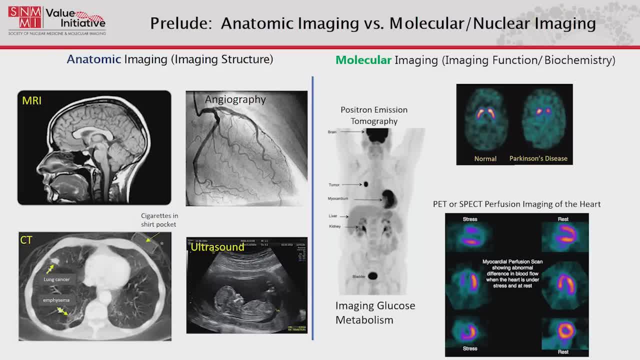 thinking. You can see the uptake in the heart because it's the muscle and it's pumping and they're using glucose for fuel. But you can also see the tumor in the lung which would just be a nodule on a CT. Malignant, not malignant, don't know, But because of the high 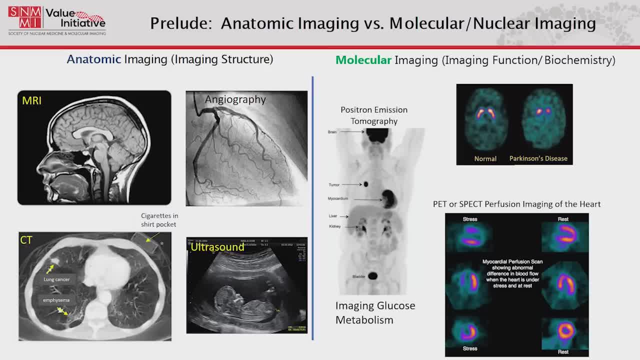 uptake. we can actually pretty carefully see the tumor. So we can pretty confidently describe that as a malignant tumor. You can see the kidney actually recognizes the radioactive glucose we injected as an imposter. So the kidney is actually filtered out and it goes down to the bladder which you kind of see down there. That's normal. 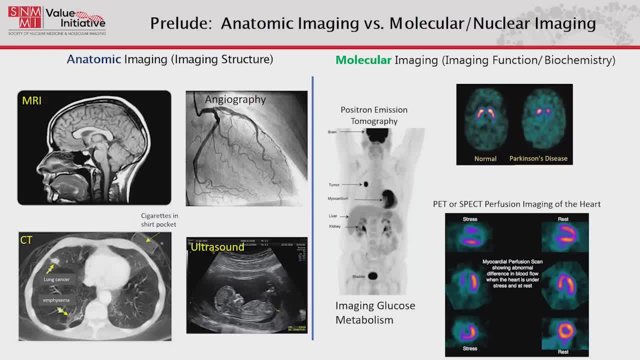 physiologic uptake. What you see in the upper right is a DAT scan. This is a SPECT scan, where you inject something that goes into the presynaptic dopaminergic system. They use this for differential diagnosis of Parkinson's disease from other motionless 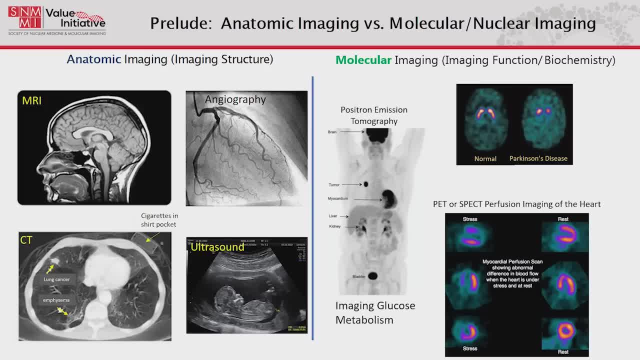 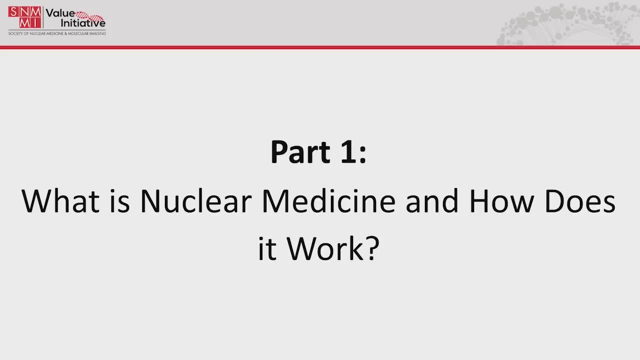 disorders And in the lower right-hand corner you see some cardiac perfusion scans that look at blood flow to the heart to look for people who have cardiovascular disease. These are just examples, but in all of these cases we're looking at the function, not so much the anatomy, which is a big 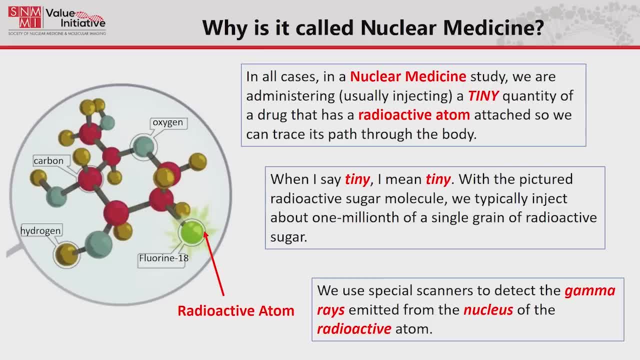 difference. So with that out of the way, we're going to get into how nuclear medicine works. So why is it called nuclear medicine? Where does the nuclear come from? Well, in all cases, in a nuclear medicine, In a nuclear medicine study, we're administering- usually injecting, but not exclusively- a tiny quantity of drug, And so in this case here's a molecule. 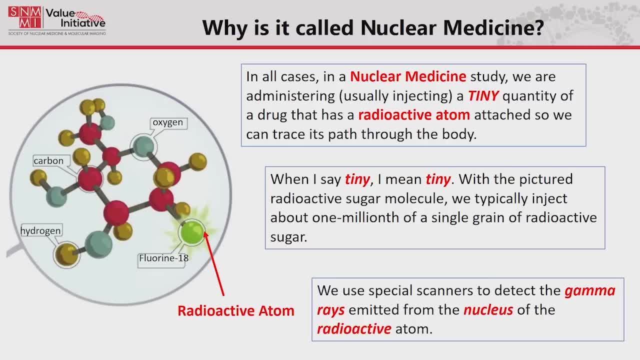 This is one of those sugar molecules, This is fluorodeoxyglucose And, right there, that's the F18. That's the radioactive tag. So my kids have one of these- It's called a cell phone- And they go around all over the country and I can track where they are because I follow where that phone is on my 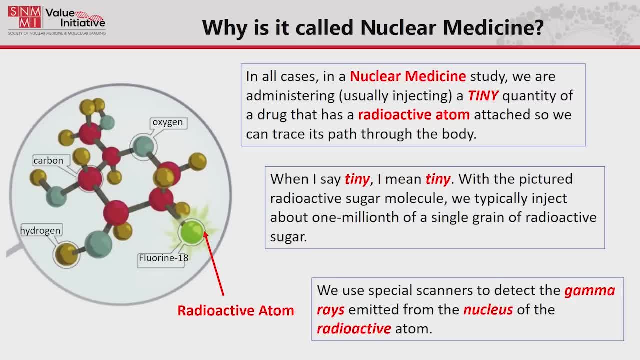 phone. Similarly, that radioactive thing that's sitting there. That's what we track and that's what we image. We don't image the molecule, We image that radioactive, nuclear- in this case fluorine-18- that's sitting there. 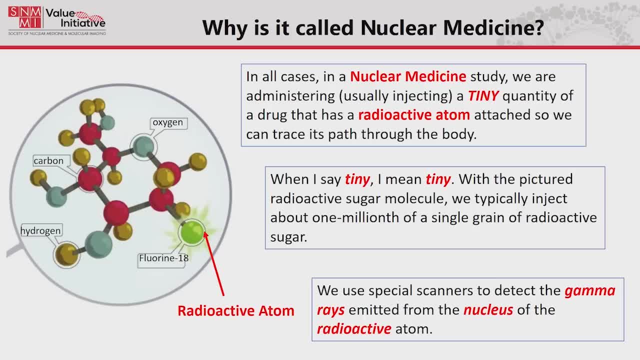 Now, when I say we're injecting a tiny amount, I mean we're injecting a tiny amount. That image that you saw of glucose metabolism: About a millionth of a single grain of sugar. That's the mass quantity of the drug. The good news is there's almost no side effects from the drug. There is radiation We have to. 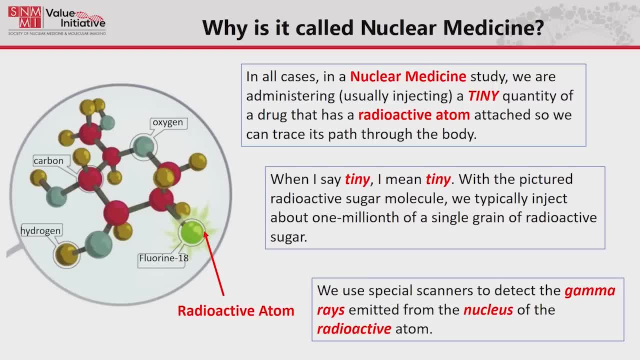 worry about that, But the of an Advil, the headache that I have right now, it wouldn't hit it at all right, So we're at subpharmacologic doses here. But then what we use is, when that radioactive fluorine decays, what we 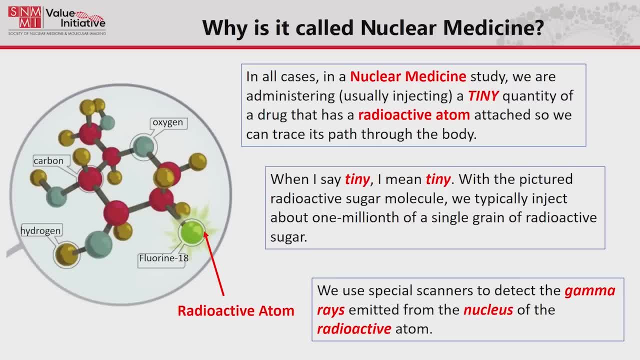 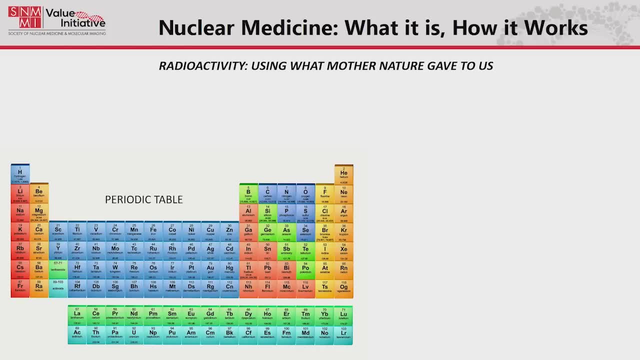 do is we get gamma rays And the gamma rays that come from the nucleus radioactively decaying, which we'll talk about in a minute. that's what we detect and that's how we get our images. okay, We're going to talk about them in much more grisly detail in a moment. 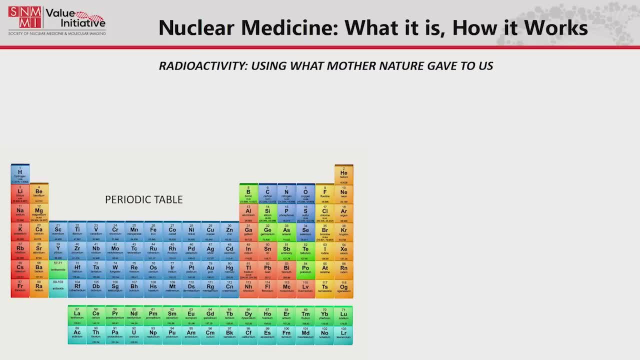 So you're probably all familiar with the periodic table here, right? And so what we do in the nuclear medicine business we use what Mother Nature gave to us. So we have these elements right, And you've all seen this. but I think I always consider the periodic table as a shallow. 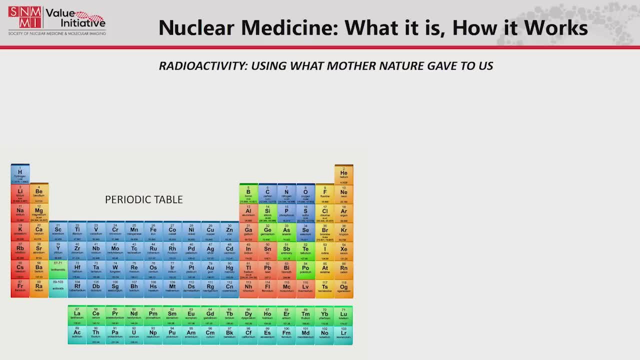 two-dimensional representation of a three-dimensional space. So if you actually look at carbon carbon six, which is, you can kind of see it going back there. carbon carbon has six protons. right, That's, by definition, what carbon is, And most of the 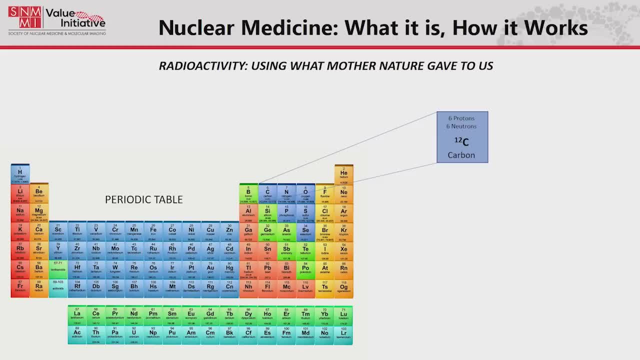 carbon in our body is actually carbon 12, because it has six protons and six neutrons. It's stable. that's what we have in our body. mostly There's some carbon 13,, six protons because carbon, and seven neutrons, which is 13,. that's stable, but only a small fraction of that. 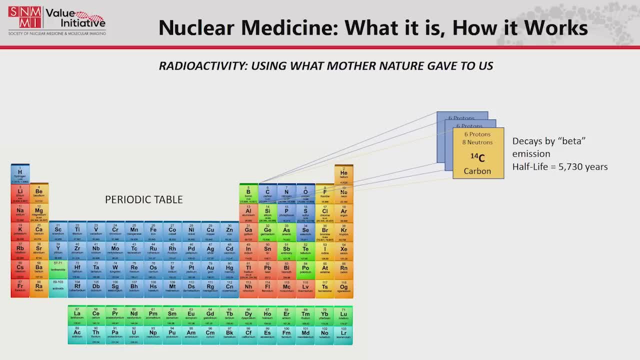 right. But the good news, at least for us in the biz, is there's also carbon 14. that has six protons and six neutrons. So we have six protons and six neutrons. So we have six protons and eight neutrons. That has too many neutrons for the nucleus' own good. It's unstable. It wants to get. 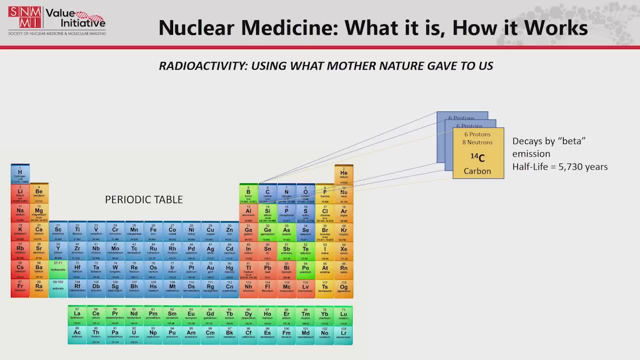 stable again, and it does this by radioactive decay. This has a half-life of about 6,000 years. We don't like to use it in people with a 6,000-year half-life, but this is what you use for carbon dating. 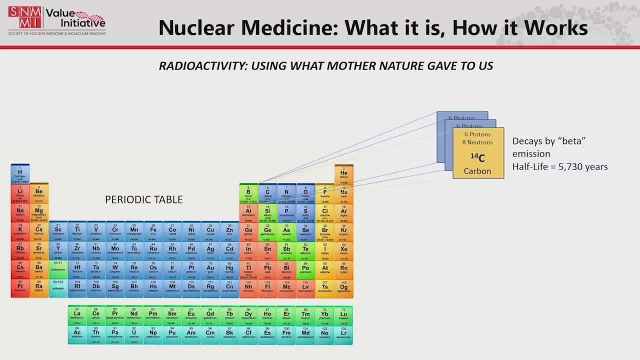 right. Mother Nature gave this to us. We have this. We can actually, and we end up using it for carbon dating. We can go the other way with carbon-11.. This actually has six protons and five neutrons. It has too many protons for its own good. It ends up. 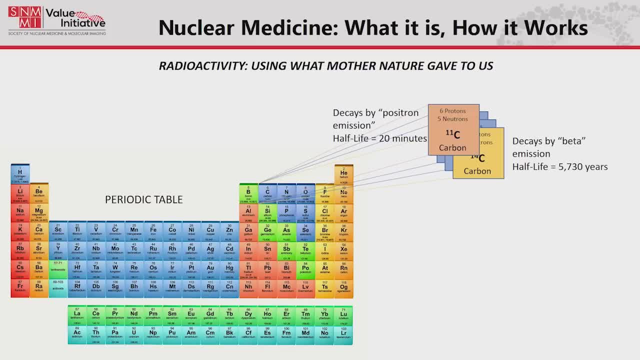 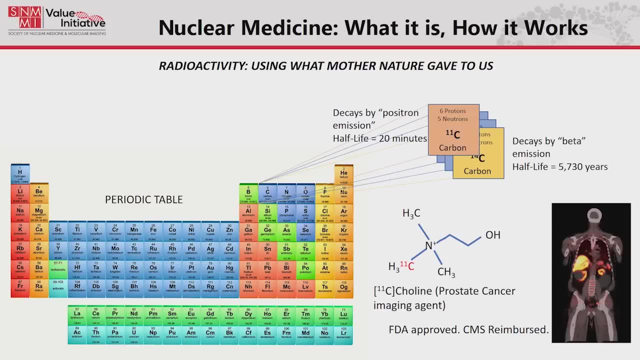 being unstable and it decays by positron decay. It's actually so unstable it has a half-life of about 20 minutes. But what we do in the nuclear medicine biz is we can take that carbon and we can attach it to a molecule whose physiology we want to trace, like in. 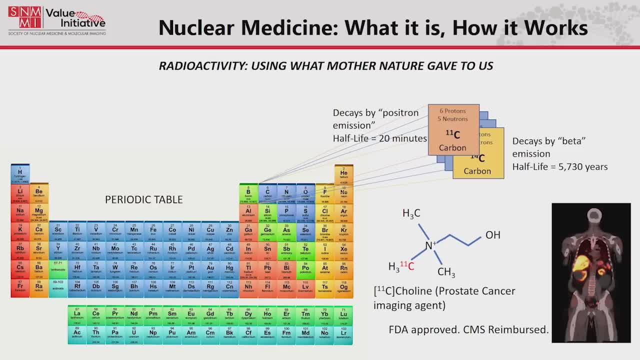 this case choline. Choline is an FDA-approved tracer to image prostate cancer And it's a little bit hard for me to point to, but kind of in the lower left quadrant there there's a lymph node down there that's actually positive for disease And on a CT we have 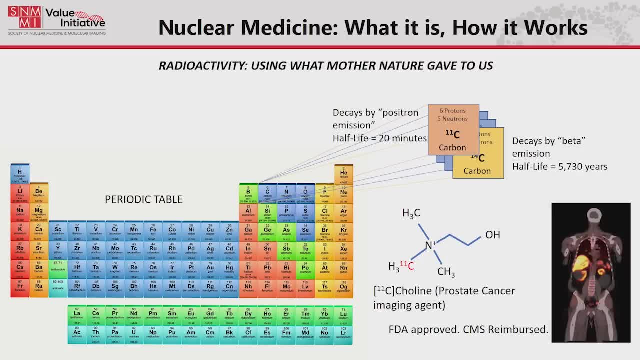 lymph nodes everywhere. You see this lymph node. It's a lymph node. It's the right size for a lymph node, along with all the other ones. It's not diagnostic but that one has cancer And that helps. It helps them guide radiation therapy or surgery or something like that, down the road. 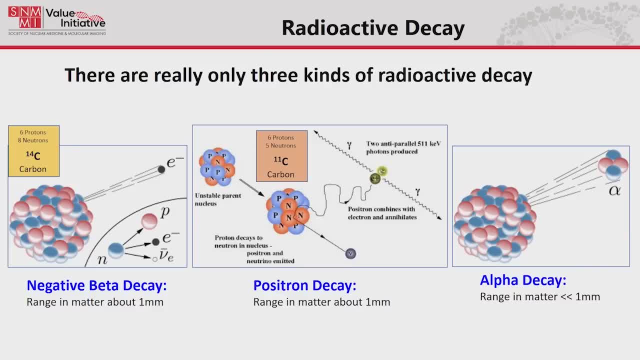 So it's the C11, but what's really important is the radiopharmaceutical there. Just another real quick science slide. The nice thing about radioactivity is, frankly, there's only three kinds we have to worry about. If there's too many neutrons in the 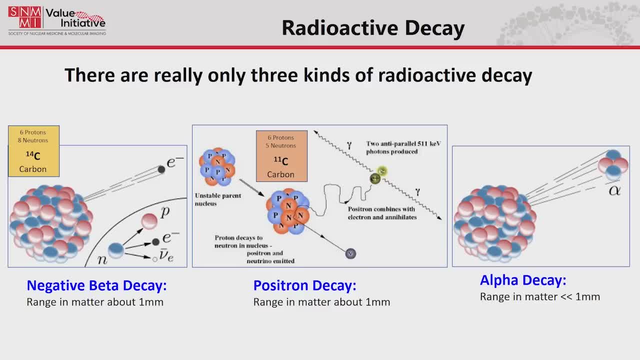 nucleus which is on the left, it decays by beta decay. That means it emits an electron from the nucleus which only goes about a millimeter. If we have too many protons in the nucleus which is on the left, it decays by beta decay. That means it emits an electron. 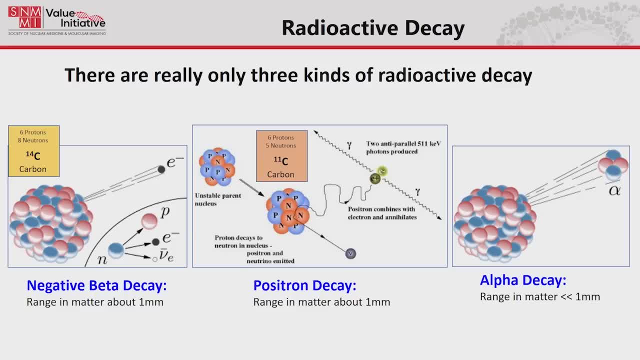 from the nucleus, That's the middle one. It decays by positron decay And when a positron gets emitted. so a positron is an electron, except it's positively charged. It's an antimatter electron. It's a real live. I mean, it's antimatter And what it does is it goes that. 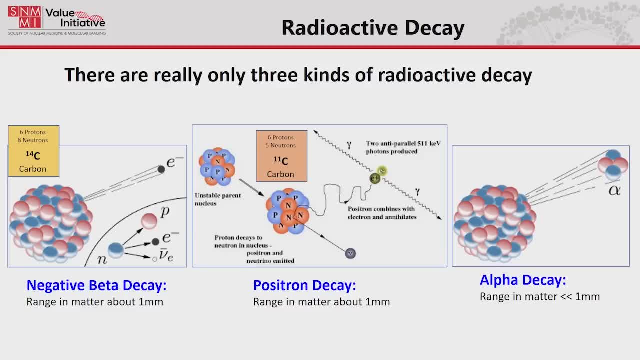 same millimeter or so until it stops. But when it stops it usually runs into an electron, because there are electrons everywhere, And when they get close to one another they annihilate That whole mass can neither be created nor destroyed thing, right. 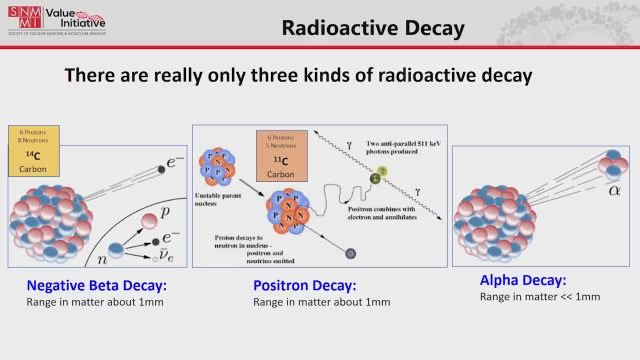 So that's wrong. The electron has mass, the positron has mass, but after they meet they annihilate, They're gone, But in their place you get two gamma rays, energy that are going off in opposite directions, back to back. That's what we detect when we do a PET scan. 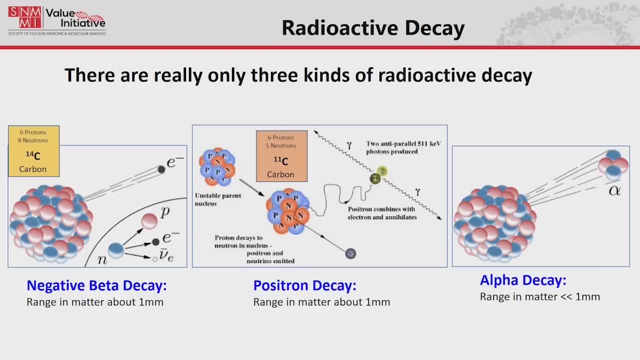 And that energy you get. that's: the E equals MC. squared thing right. The M is mass, the E is energy. And then on the right side that we don't use so much for imaging but we use for therapy, we have alpha decay, where the nucleus emits this very massive it's like. 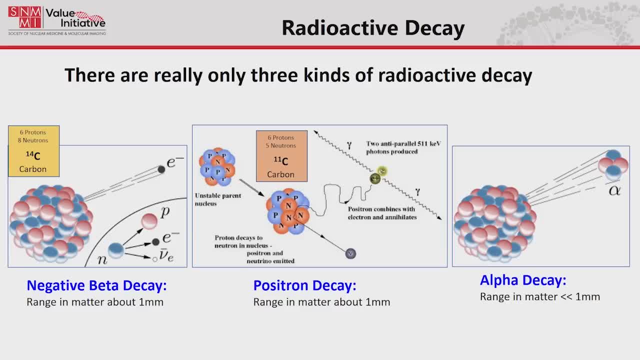 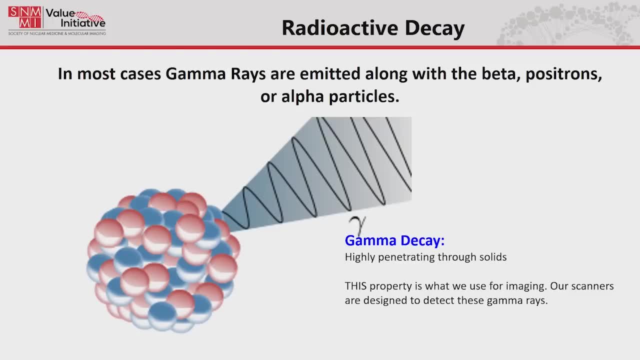 instead of emitting a ping pong ball, it's emitting a bowling ball, And that ends up being important when we talk about therapy a little bit From an imaging standpoint, what's important is with the alphas and with the betas and, frankly, with the positrons as well. see, we can't detect the beta particle, It's only. 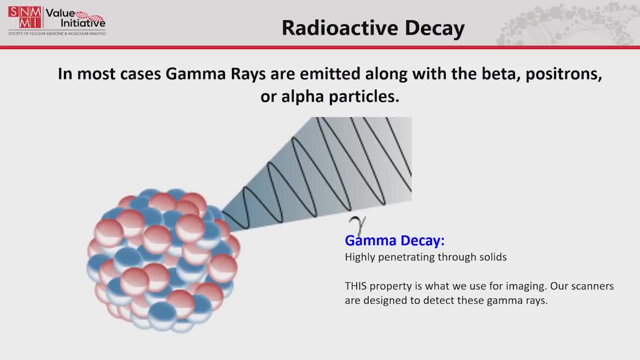 going like a millimeter. It's going to stop in the body. Same thing with the positron, But usually what happens is, after it emits that beta particle, the nucleus is in an excited state and it goes to the ground state And when it does that it emits a positron And 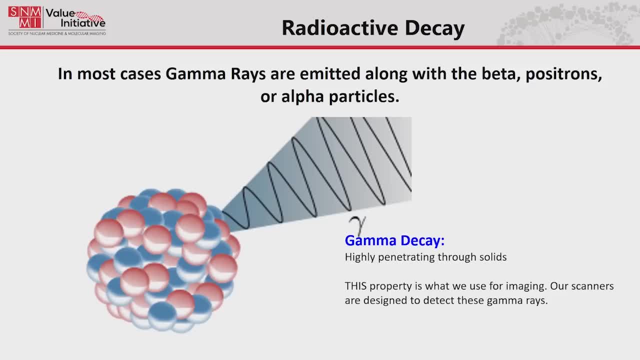 it emits a gamma ray. The gamma ray is a high energy electromagnetic radiation and it can go through the body, And this is what we're detecting When that nucleus decays, by whatever it does, it emits this gamma ray and the gamma ray can go through the body. 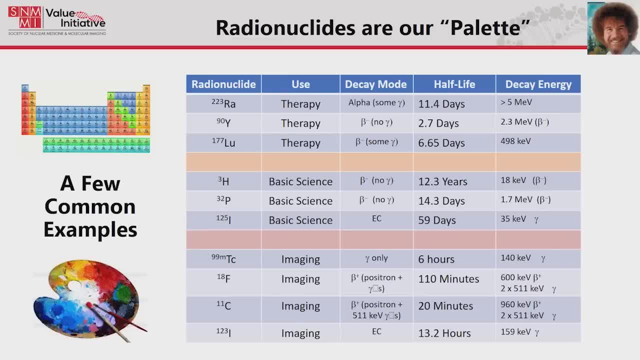 and we can detect it with our scanners. This is my tribute to Bob Ross. Most of you who know Bob- even my kids- know Bob Ross- He's kind of a superstar now, even for them. So we use these radionuclides that are available to us. We use these radionuclides that are 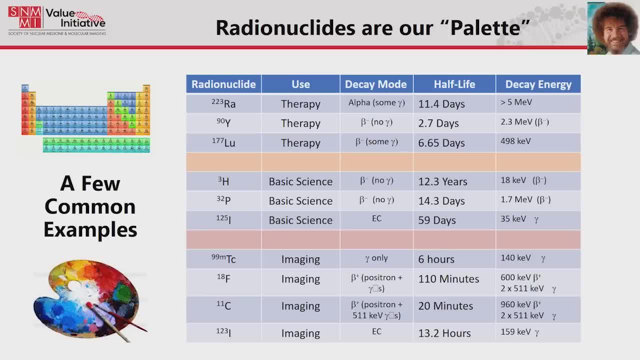 available to us, kind of as our palette. We like to choose the ones that fit our needs for imaging or therapy. This is just a list of 10.. There's probably about 60 or 70 useful radionuclides out there. Some of them have short half-lives, like the imaging ones We'd 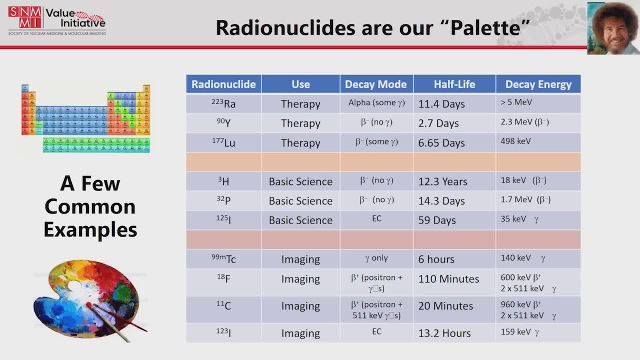 like to inject the short-lived ones for imaging, because then they'll just go away By the next day. they're pretty much gone For the therapeutic, which is kind of up at the top. if we're going to inject therapeutic radionuclides, we'd like to have them sit. 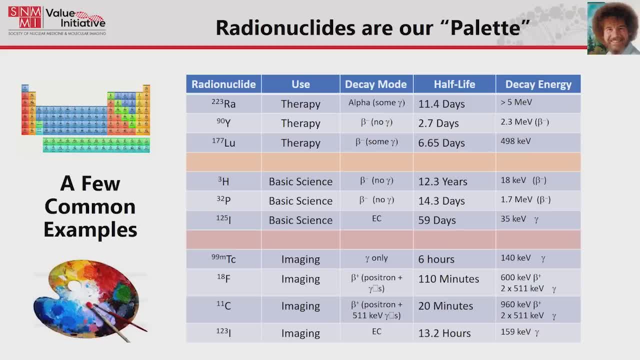 there We're bombarding the tumors for a really long time. We'll get into that. So having a longer half-life is a good thing, And the kind of decay, all these things enter into it. We have to get very clever about how we use them. But it's not just the radionuclide. 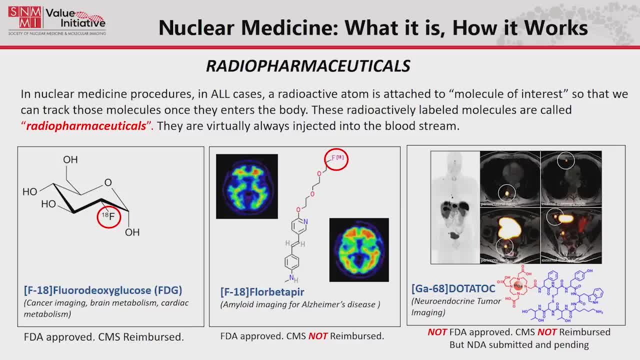 It's not just the half-life, Really, it's all about the molecules we attach them to. This is just three of several hundred that are out there. Most of them are on the research phase. Some of them are FDA-approved. Some of them are FDA-approved and we use clinically. Here's three that are out there. that all kind. 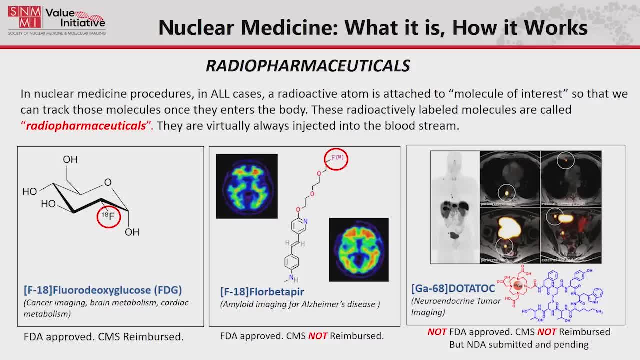 of represent different things. There's that glucose, one again that has fluorine-18, has a half-life of about two hours. decays by positron decay. Actually, all of these are positron emitters. The one that's in the middle is fluorobeta-pyr, which we use for 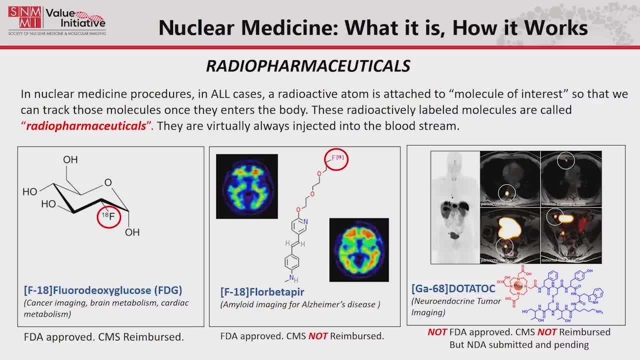 Alzheimer's disease. What's interesting about this is it does a great job of attaching to the amyloid in the brain for Alzheimer's disease, And it's FDA-approved And CMS doesn't really reimburse for it. And then, on the right-hand side, we have Gallium-68-Dota-Toc, which is very much like NetSpot for those of 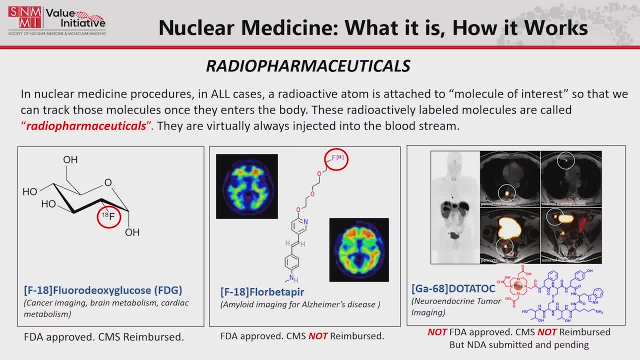 you who are familiar with it, which is approved. Gallium-68-Dota-Toc is not yet approved, although we at the University of Iowa have submitted a new drug application And hopefully we're about two weeks away from approval for that. So fingers crossed on that. 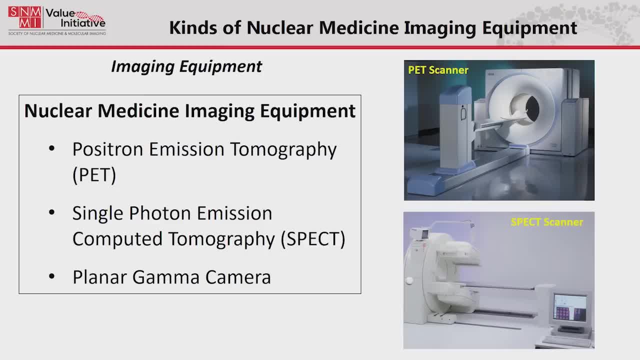 Yes, What CMS is? Oh, I'm sorry, When I say CMS, I mean Medicare, right? So Medicare has chosen not to pay for those Alzheimer's because we don't really have a treatment for it, right? So they say: oh, you diagnosed. 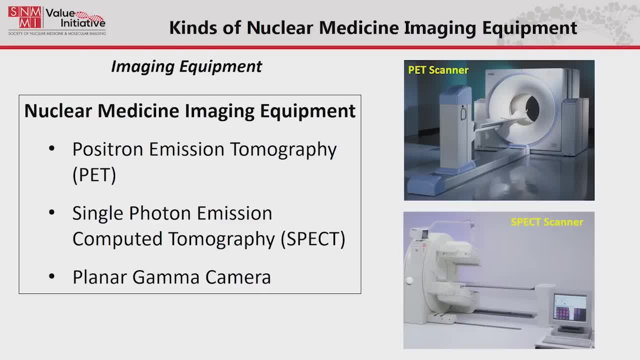 it. so what? That's their point? I don't necessarily, So bottom line here is: So what we do is we have these radionuclides that are attached to these radiopharmaceuticals, We inject them into patients and then we have to image them. 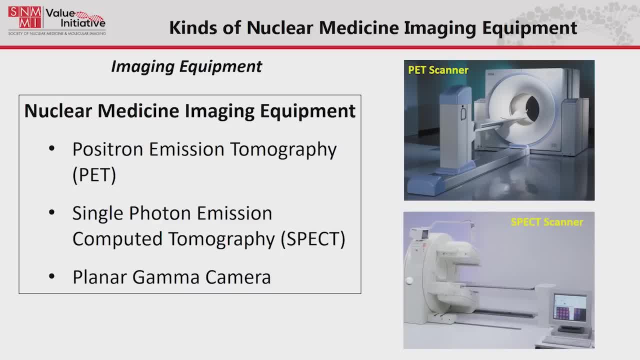 So if they're positron emitters, we use the PET scanner. It's designed to get both those. So we have a ring of detectors. It's designed to get both those gamma rays off of it detected at the same time If they just emit that single. 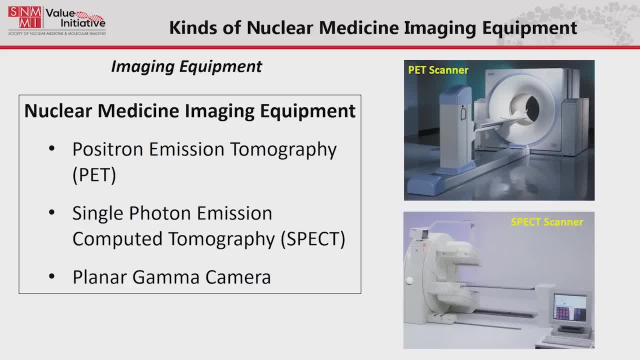 gamma ray, then we use the SPECT scanner which is down below, And so that's usually the beta emitters we use SPECT scans for And the standard planar gamma camera images. we generally use the same SPECT scanner which is down below. The procedure is pretty simple. 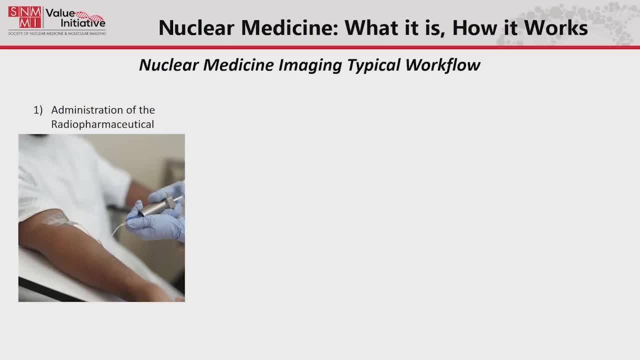 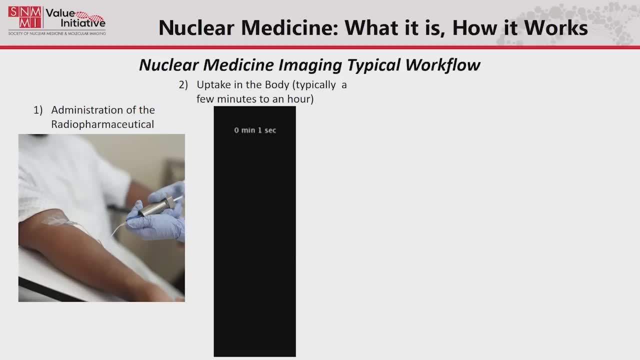 In general we administer radiopharmaceutical. 90, 95% of the time it's by injection, but we do have other modes of administration, So I'm going to show you this. This is. some friends of mine work with a company. 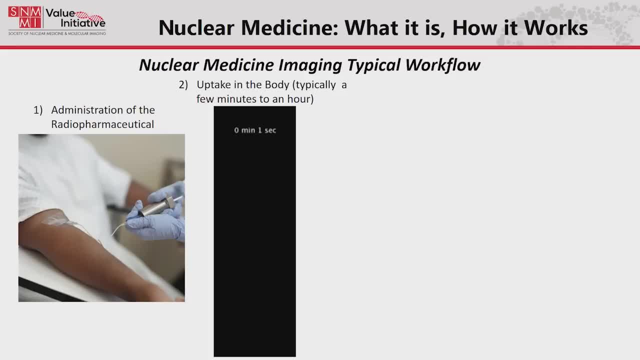 in China and they built a PET scanner that's two meters long so you can get the whole patient in there at the same time- And this is one of the very first images that they Let me see. if I can get my Very first images- they injected FDG in the leg and this is one-second images. 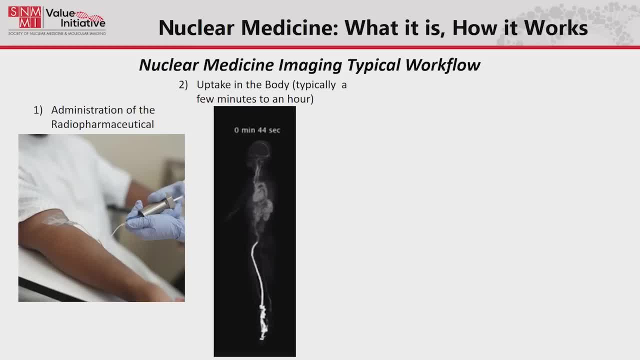 You can see it going up the leg into the lungs, into the brain- We're about 45 seconds in. It's beginning to distribute into the heart, into the liver, et cetera, And now it's kind of going two. 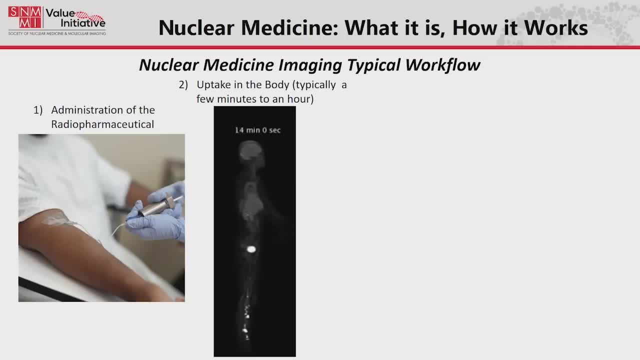 minutes. You can see it going into the brain as it's being metabolized. You can see the kidney has actually filtered out and the bladder is filling up. You can see all this over time. First time we've ever been able to see what an injection does all at once, let alone what FDG. 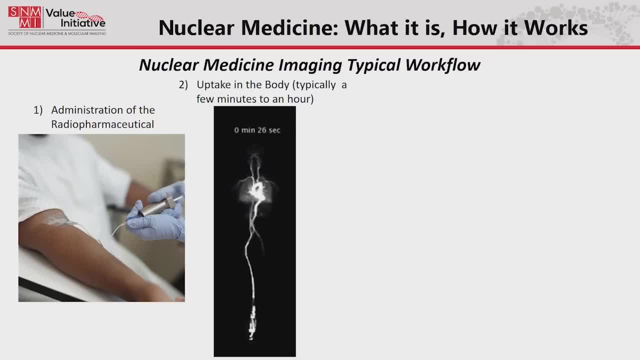 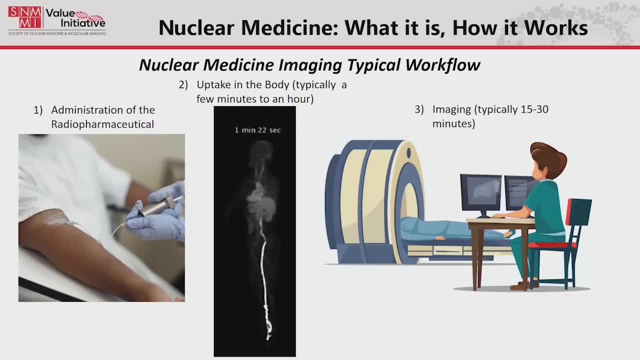 does So we can get full pharmacokinetics of all of these things now with this new device, PET scanner, but two meters long. Very cool Bottom line is: we do inject this stuff. There's an uptake period. That uptake period could be anywhere from a few minutes to maybe an hour or 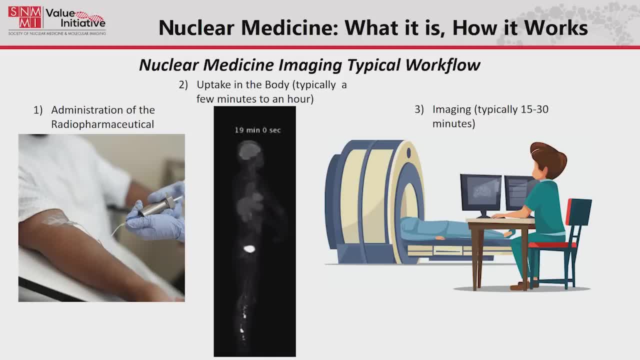 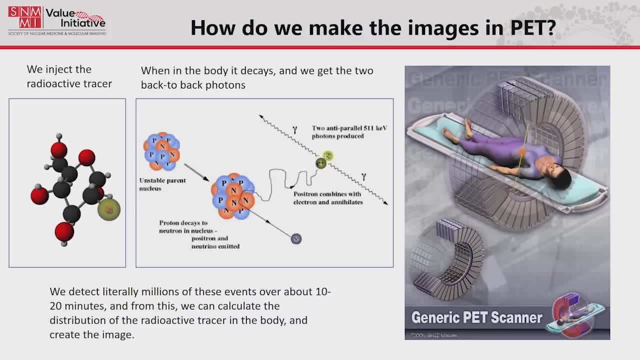 two. When you put them in the scanner, the scan typically takes 15 to 30 minutes. Actually, these days, with new scanners, it's usually down to 10 to 20.. You can get a whole body scan. So that's how we do it. Now the question is: how do we get the? 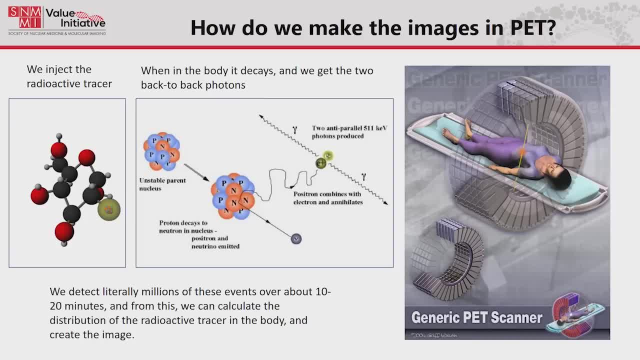 images. Just a couple of really quick slides here. Once again we have our glucose molecule that actually has the unstable nucleus When it decays. once again we have that positron that goes off in about a millimeter. We get the annihilation, And then we have those rings of detectors. 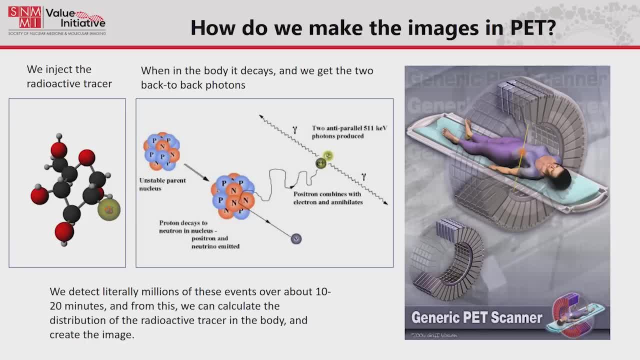 which actually try and detect both those photons at the same time. At the same time we can actually detect the photons within about five billionths of a second of one another. We can actually kind of trace back to where the event occurred, because two points define a. 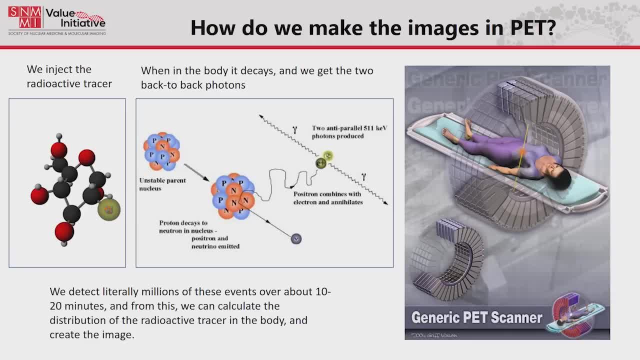 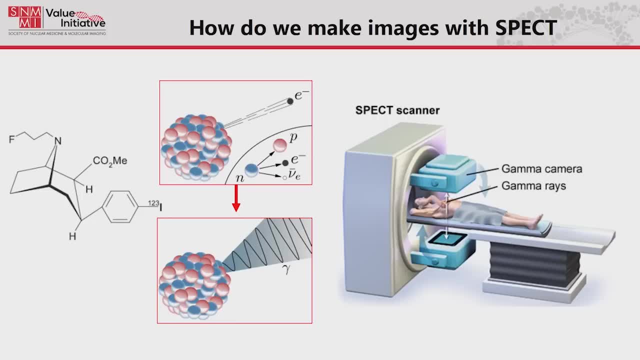 straight line. We don't just detect one of these, We detect tens of millions of these events And from that we can reconstruct these images. So in PET we're looking at two photons at once In SPECT. so this is DAT scan. This is the one that looks for Parkinson's disease. 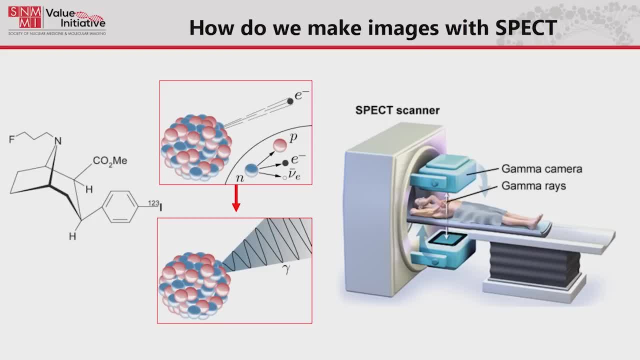 It has iodine-123, which has a bit of a longer half-life, But when it emits that beta particle. but then the important thing is it emits that single gamma. There's two detectors, one on the top and one on the bottom. It detects if it's going up or going down. We actually detect. 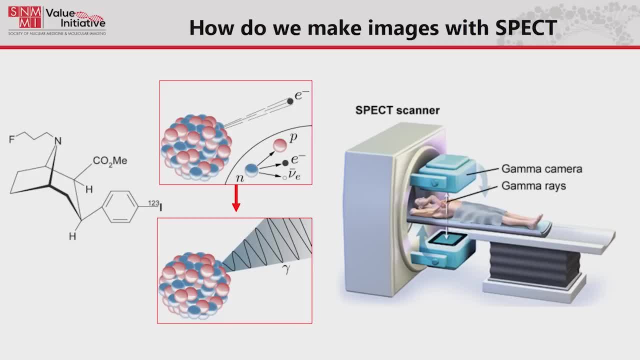 it And those detectors actually rotate around the patient over time. It goes about a half revolution And from that we can reconstruct what the distribution is in the brain, or really wherever, or the heart, or whatever it is we're looking, And that's as much as I'm going to go. 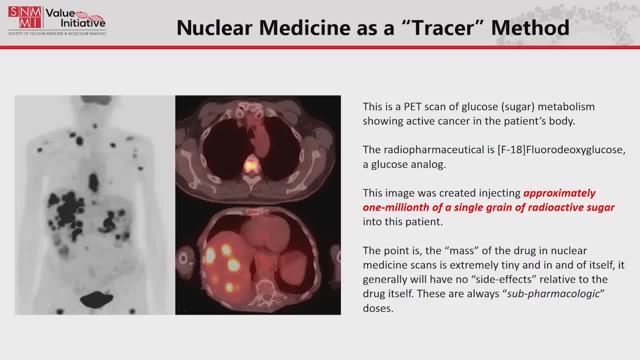 into how those scanners work. I just want to repeat again that nuclear medicine is always tracer methodology. The quantities, the mass quantities that we inject are really really small For the most part, although FDA doesn't like us to say it. 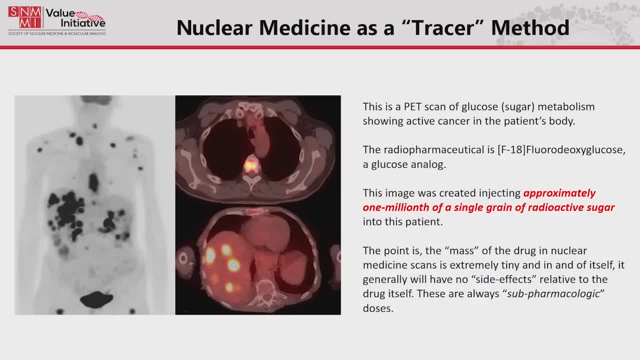 there's really no side effects associated with these quote-unquote drugs because the mass quantity is so small. That doesn't mean we don't have to worry about the radiation dose. It doesn't mean you don't have to worry about- ooh, there might be. you might get a bruise at the injection. 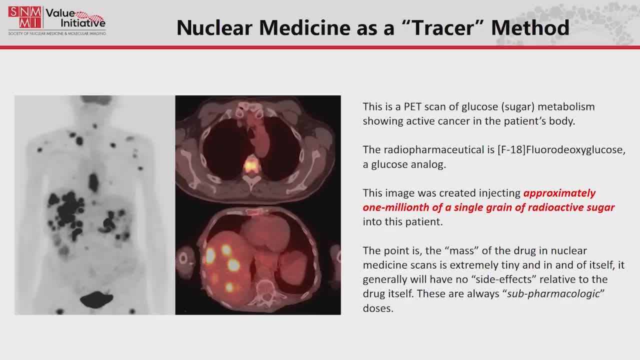 site. But the drug itself, the mass is so small we really don't worry about that too much And FDA realize they make us check it. but they realize that these are really low-risk drugs from that standpoint. It's not like you're giving a therapeutic drug for these diagnostics. The mass: 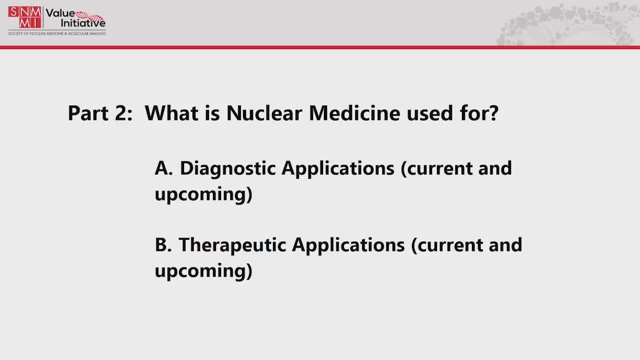 is really small. Okay, So now that's how this all works. Let's go to some of the applications. I'm going to talk about the diagnostic ones first, the current ones, and then some of the unapproved ones that are coming down the pike. 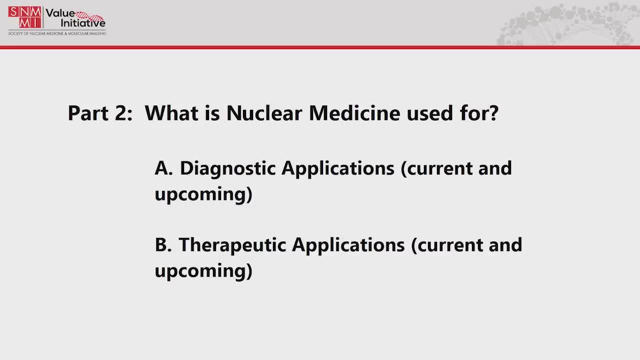 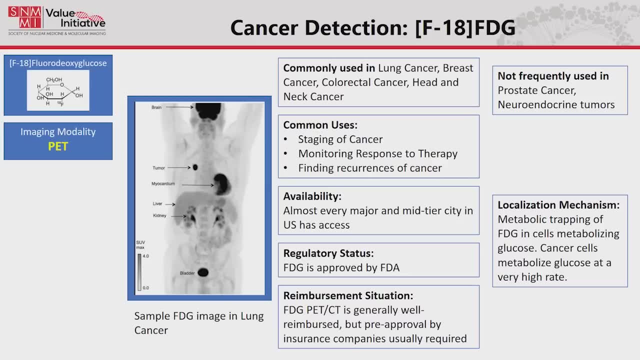 Each of them. this is by no means an exhaustive list, It's just a sampling. I think I go through about 10 or so, And then I'm going to go through a couple of therapeutic applications and then on into safety. So all of these slides coming up right now have the same format. You've seen the 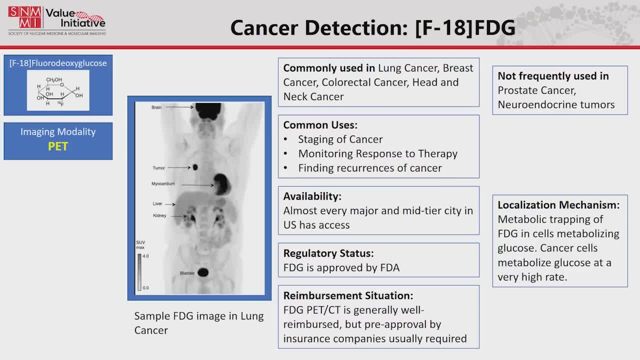 FDG ones. I'm not going to go into too much detail here, but I am going to go with the format. So in the upper left-hand corner is the molecular structure. I know you can't see it very well and frankly I don't care. What I want you to realize is they're just all different. 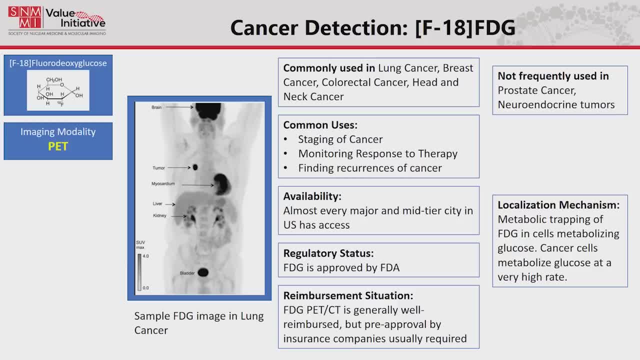 Whatever the application is, the molecule has to be tuned to the physiology that we want to trace. I have the modality, whether it's PET or SPECT or standard nuclear medicine. I have an example, what it's used for, what its availability is and the regulatory and reimbursement situation. 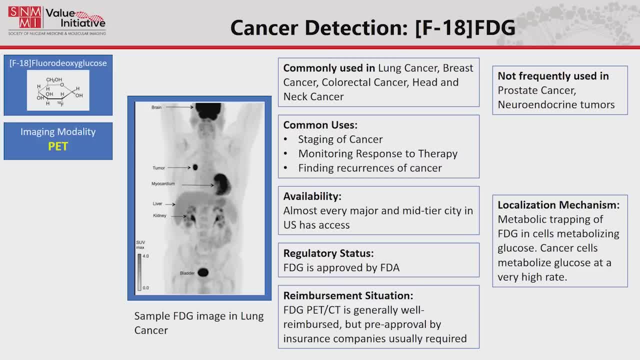 And then, almost most important, is the localization mechanism, why it does what we think it does. So this we've talked about fluorodeoxyglucose. It's used for a wide array of solid cancers, solid tumors, but it's not used very often, at least for prostate cancer or 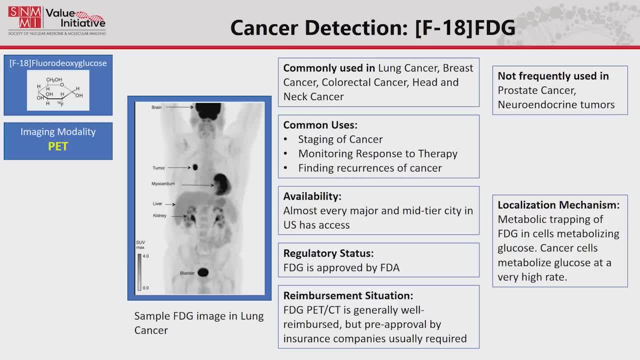 neuroendocrine tumors. Those are relatively indolent. They don't usually grow very fast and as a result, the glucose uptake they don't require a whole lot of energy, so they don't show up very well. So we have to be a little bit discriminating how we use it. It turns out that 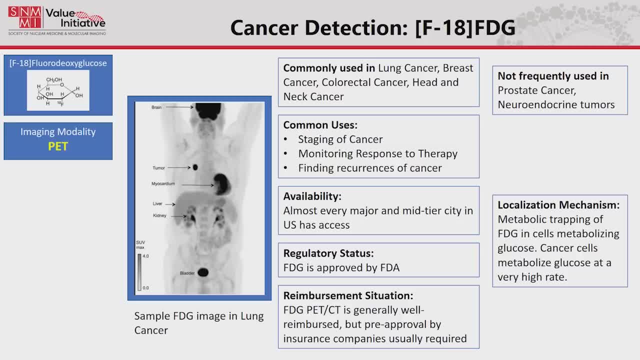 most cancers use glucose like crazy, which is why they light up like little Christmas lights kind of all over the place, because they've actually got something wrong with their metabolism that makes them burn glucose. It's approved, It's available just about everywhere in the USA. 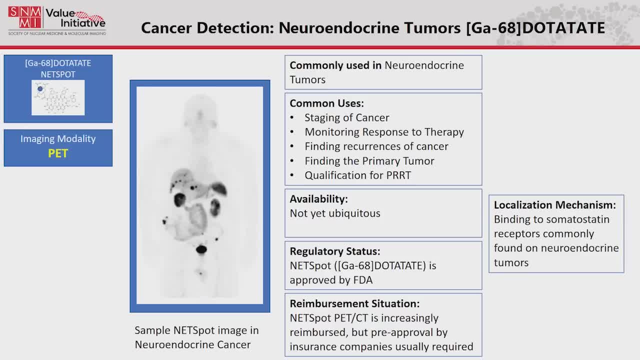 This is NETSPOT gallium-68-dota-tate. It's a much more complicated molecule. Gallium-68 has a half-life of about an hour. It's used specifically for neuroendocrine tumors. Why is that? Because 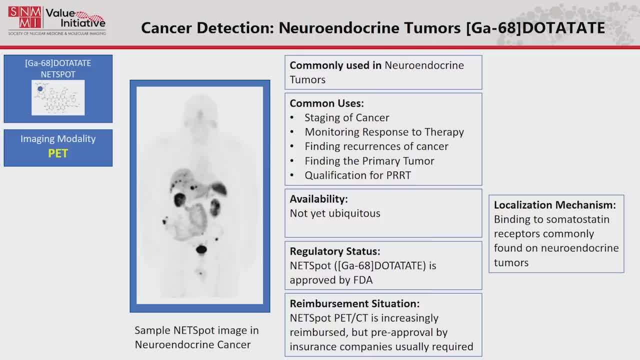 neuroendocrine tumors overexpress somatostatin receptors commonly found there, and so they've been clever enough to define a drug, a molecule, that seeks this out and binds to it and actually sticks and pretty much won't let go. And that's what this NETSPOT, this gallium-68-dota-tate. 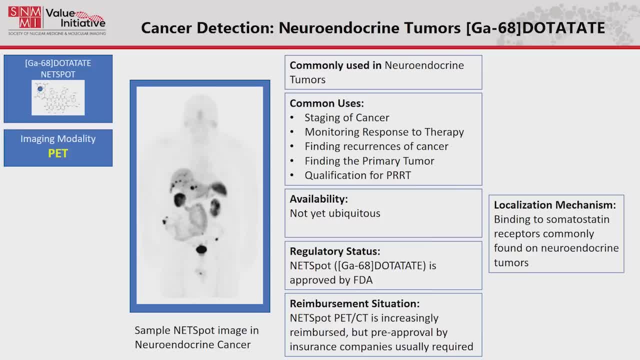 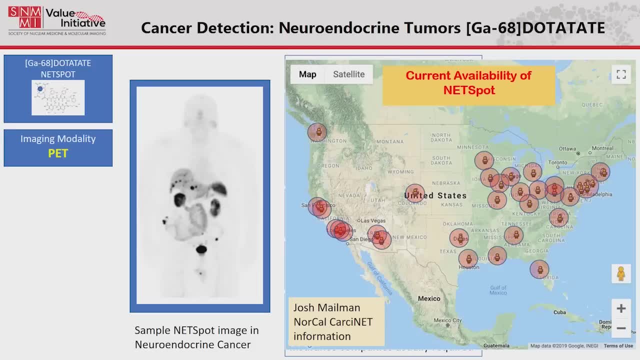 does. It is approved. It is reimbursed. although you have to get preapproval by insurance companies, It is not quite ubiquitous. as far as availability is concerned, and I think this is a modification of something from Josh's website, where he has the sites where this is produced- His doesn't have little circles. I have little circles that. 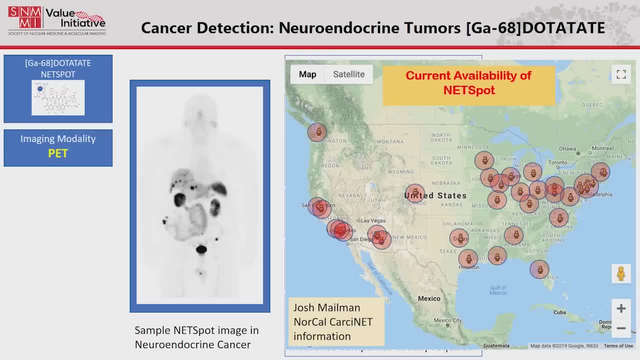 define about a one-hour radius around these, because it only has a half-life of about an hour and you don't make much of it when you do a synthesis. So these are the places. you have to be kind of within one of those circles in order to get this, because it's not widely. 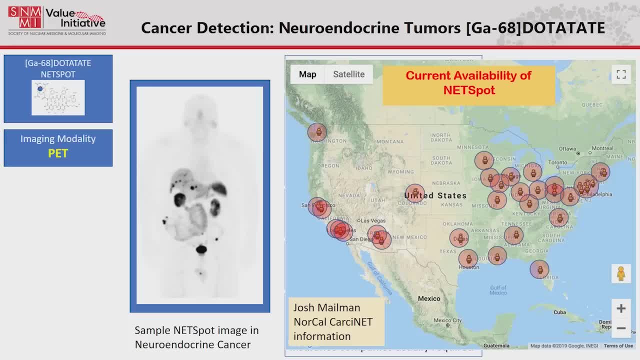 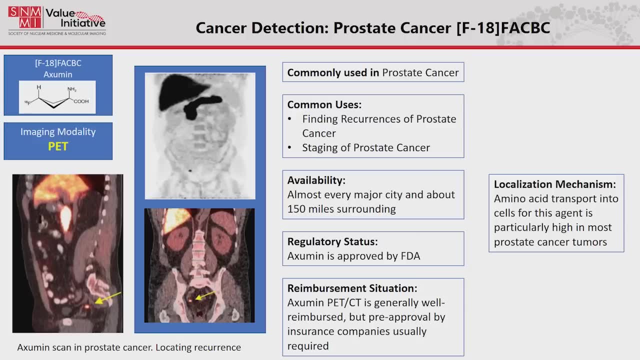 distributed, But the good news is it is available. Okay, so on to prostate cancer. So I got a couple of, so I showed choline before. That's one approved agent. Another approved agent is F18FACBC, which has the trade name axiomin. It's for prostate cancer. This is an amino acid. 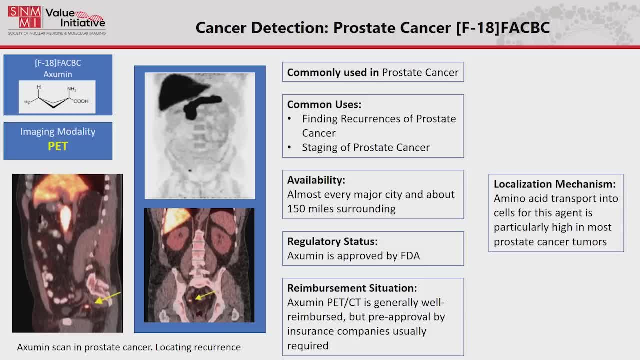 and it targets a transporter that is overexpressed in prostate cancer, And here you can see in this image the little dot there in the pelvis which is where it's spread to, which is very helpful for the physician to either do surgery or radiation. 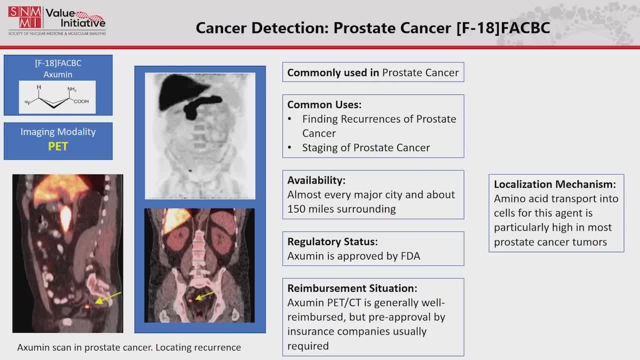 therapy to make sure he targets it. This one: I made a point of showing the CT background and those color ones right. So sometimes the PET scans are so specific you can't see the background anatomy so the surgeon doesn't know where to go because there's no landmarks. So most PET scanners 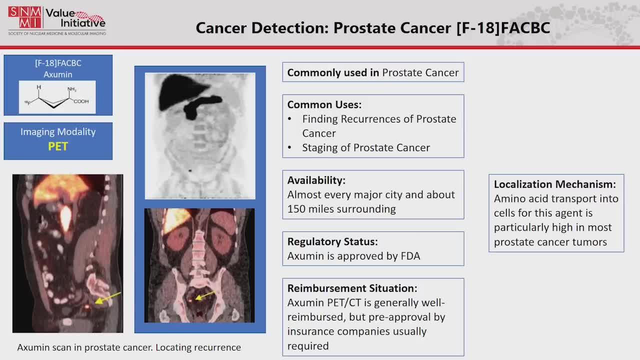 really all PET scanners. these days you can get a CT done at the same time, so you have the anatomical backdrop in which to project the PET scan, so you know exactly where you're looking. This, once again, is available just about all over the country, because you can get it in the 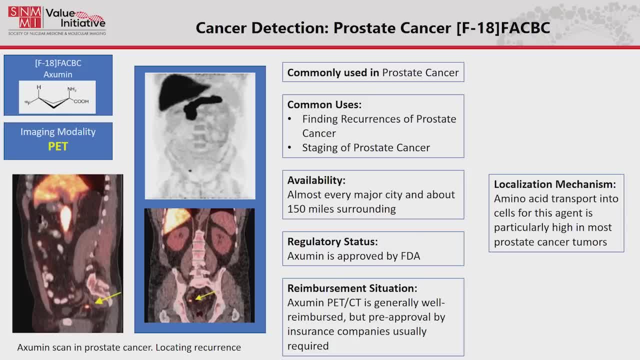 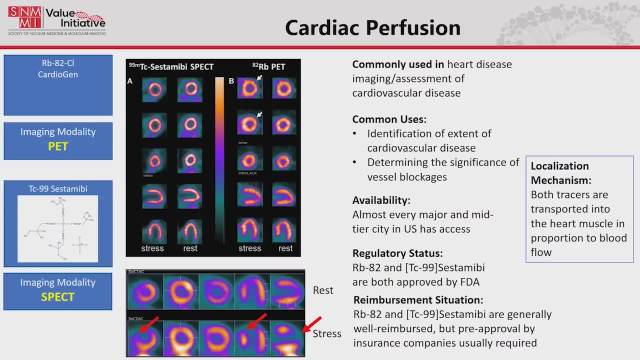 US because it's transportable. You can go on the order of three hours outside. The reimbursement situation is good, but pre-approval is required- Cardiac perfusion. So I have two examples here, both PET and SPECT. They do pretty much the same thing. Perfusion means how much blood is going to. 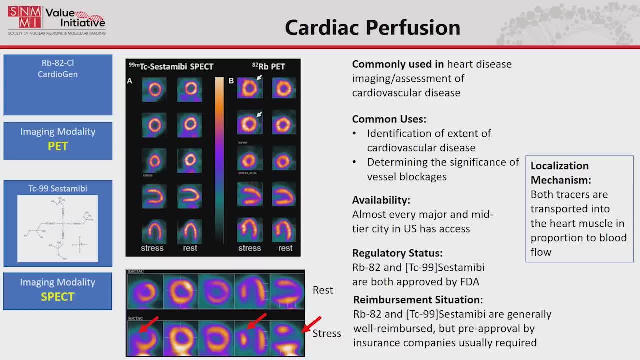 different parts of the heart. The left ventricle is the important one here. This is what pumps it all the way through. That's the big muscle, muscular part of the heart, And it's kind of shaped like a bullet, And so it's a little bit like a bullet, but it's a little bit more. 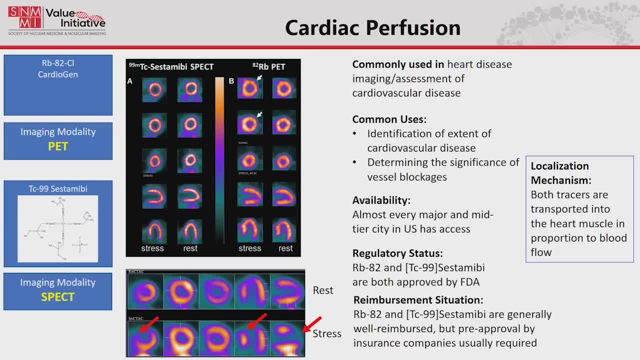 like a bullet And so where you see those round doughnuts, that's like looking at cross sections of the bullet, And what you like to see is like what you see assessed to maybe SPECT scan on the right, the rubidium on the left, the rubidium on the right And what 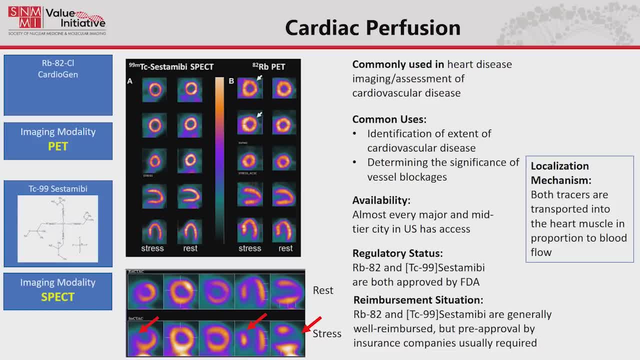 you like to see is that nice round doughnut there. The ones below it that look like this is a vertical slice through it. The one on the bottom is a horizontal slice. Once again, those are normal. Not normal is what you see down below. The apex is the tip of the bullet. 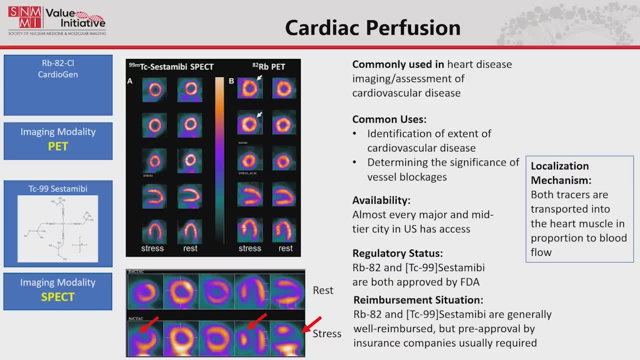 And you can see under rest conditions at the tip it's pretty much thinned out. That means there's probably a stenosis, not a whole lot of blood getting there, And under stress conditions they get on a treadmill and they inject it. You can see there's almost no blood getting. 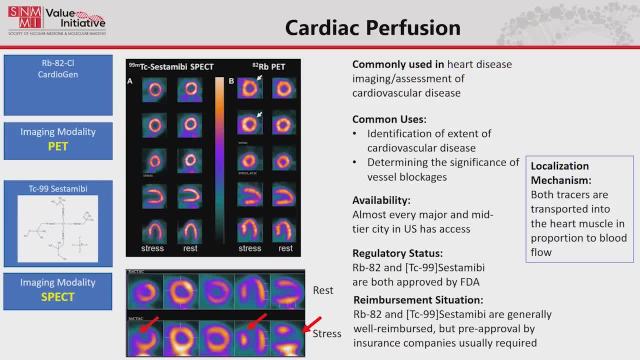 there because the stenosis is so much. When people have angina, they have pain, heart pain when they exercise. This is what's happening. That heart muscle is not getting the perfusion. They can see the extent of it and the impact of stress on it with these cardiac perfusion. 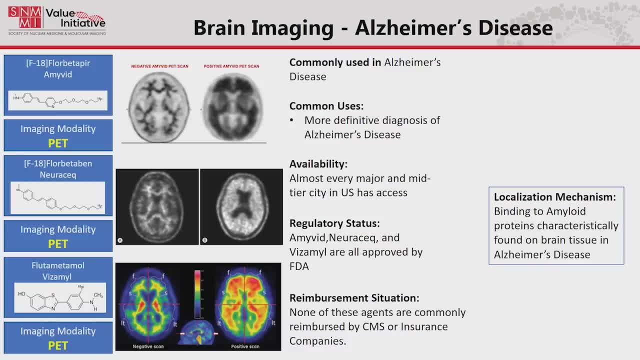 I mentioned this brain imaging before. Drug companies were all hot on this because they found a way to image the amyloid. Three companies went as far as to get these approved. None of these are reimbursed. All of them are approved. They are available. They're being used extensively. 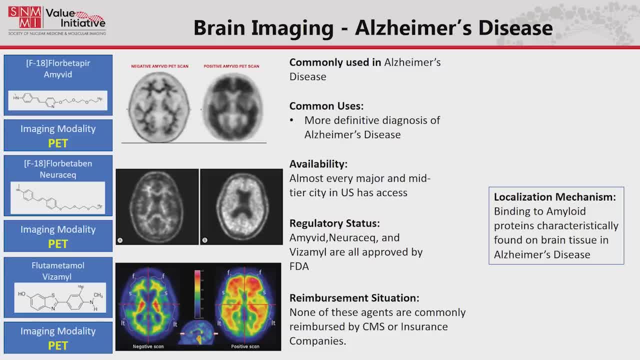 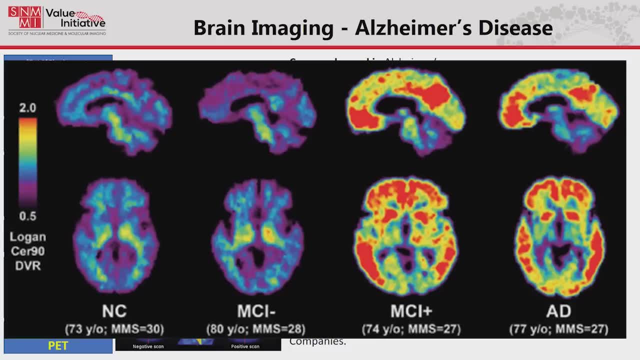 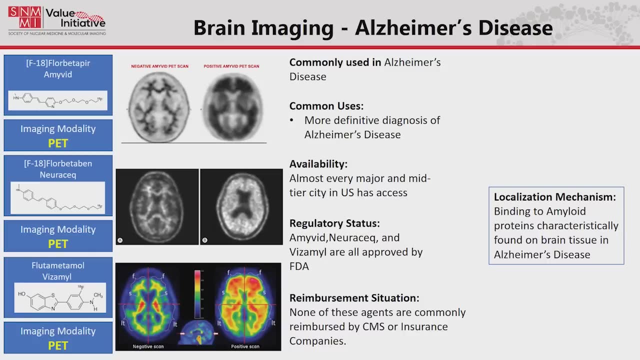 in clinical trials, Largely to look at treatment drugs, because they like to know whether somebody actually has Alzheimer's disease or not before they actually try the drugs. This is an example of kind of how it works. I should go back and say the ones on the right. I'm sorry. I'm sorry on the left is what. 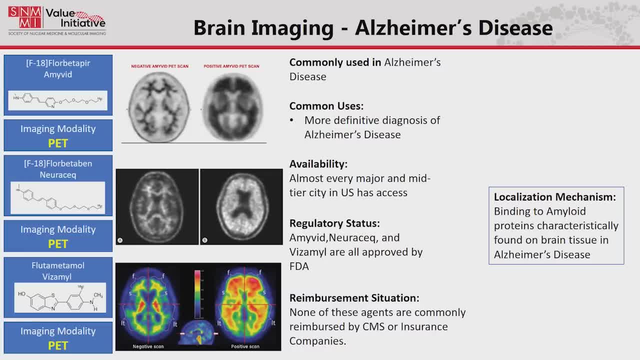 normal uptake is, That's white matter uptake. But when you start developing amyloid plaques on the cortex, which is the outside of the brain, that's what you see on the right-hand side. They all they look a little bit different But in all cases you see that the amyloid 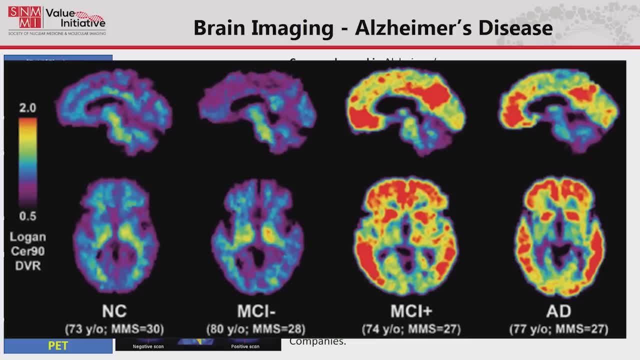 spreading to the outside. Where this ends up being important is in a series like this. These are four different patients: The one on the left, the one on the right. the one on the left is normal. The two middle ones are the important ones. MCI stands for mild. 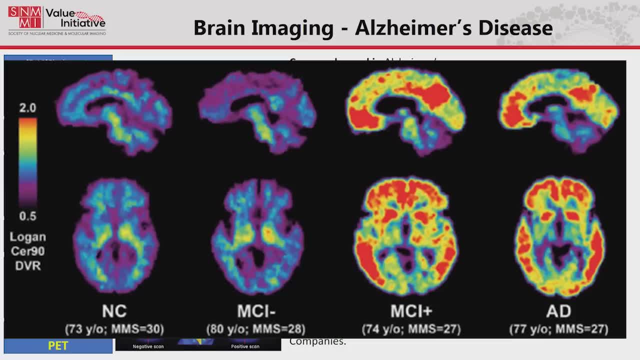 cognitive impairment. That means you're a little bit forgetful. You forget what you said five or ten minutes ago. But there's a lot of causes for that and it could be early on. These two middle patients have the same symptoms. One of them doesn't have Alzheimer's. 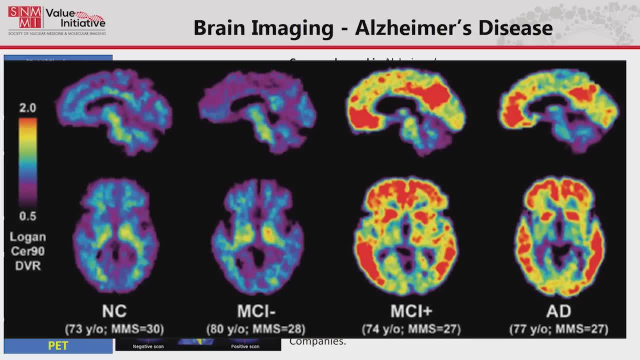 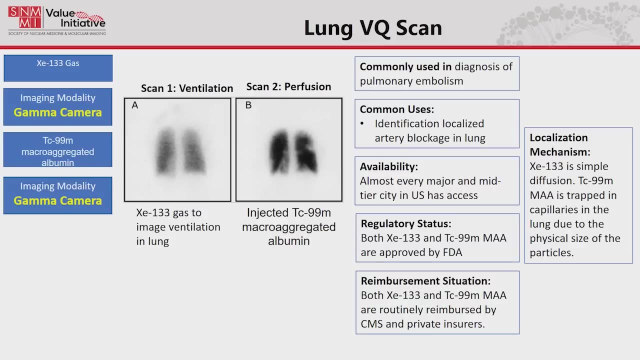 disease, The other one does. You can see the mild cognitive impairment amyloid burden is pretty much the same as full fledged Alzheimer's disease. That's the AD on the far right. So differentiating it is actually pretty important, but CMS and the Medicare people don't seem to think it's that important yet. 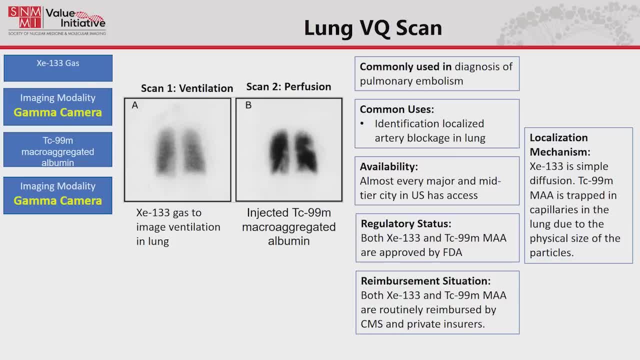 I only do this one. This is a bread-and-butter nuclear medicine scan. This is actually not SPECT, This is just planar. I bring this up because I mentioned different kinds of administration. So the ventilation scan is done with xenon-133, which is radioactive gas. You inhale this, So 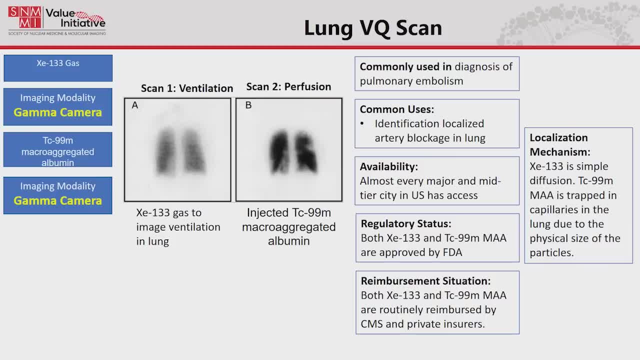 that's what you see on the left-hand side. That's just to see where the air is actually getting in the lungs, because sometimes those are not normal. What you see on the right, they use this for identifying pulmonary embolisms. Those should be kind of uniform. 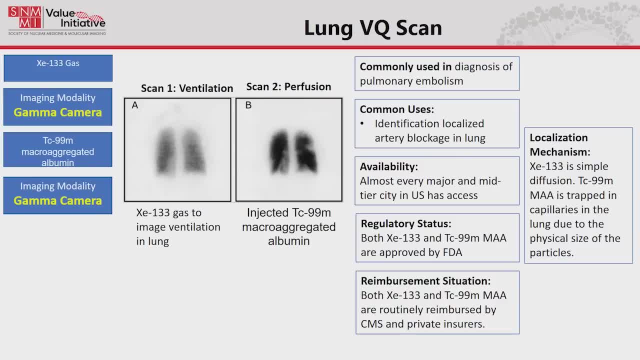 lung, kind of black on either side. This is actually looking at where the blood goes, because it's not just where the air goes. The air has to go through and get into the blood. Where you see those inhomogeneities, where it's light in there, that's where the blood. 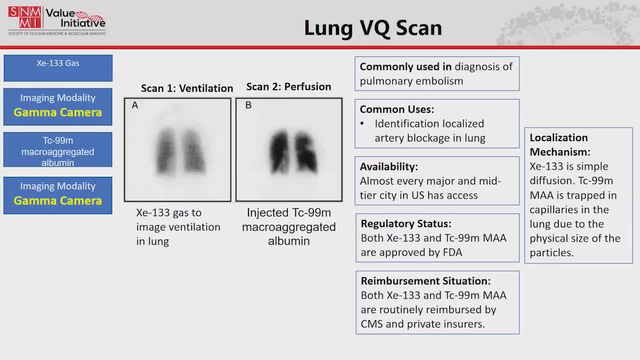 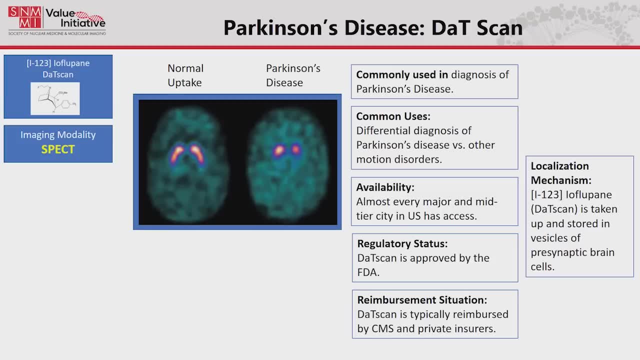 starts to get in. So that's what you see on the left-hand side. It's not getting where it's supposed to. This is a standard nuclear medicine scan done with two different drugs, one xenon, one technetium-99 labeled. I mentioned and showed. 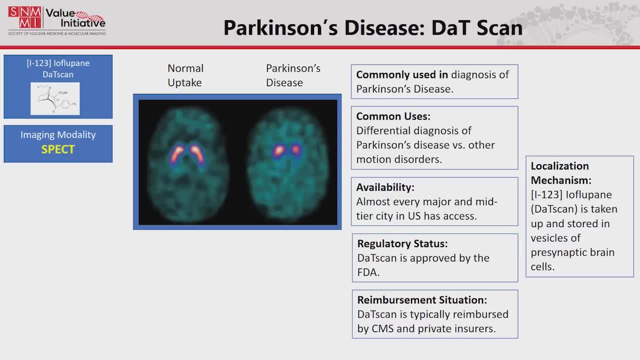 this Parkinson's disease one, this DAT scan. This is an approved agent, iodine-123.. It's SPECT And this is taken up and stored in the vesicles of presynaptic brain cells which are generally sitting in the caudate and the butamine, which is those comma-shaped things on the left. That's. 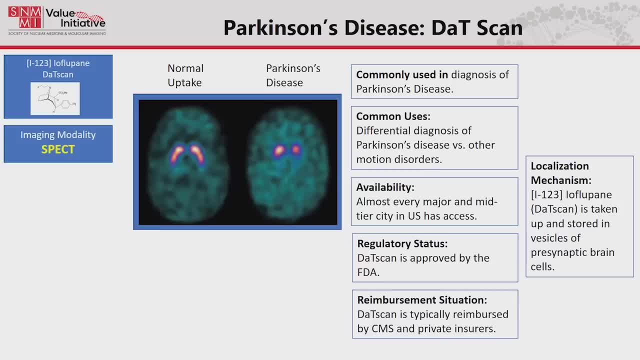 normal, The butamine begins to the cells begin to die and then in Parkinson's disease, And so you can see on the right-hand side the tails have kind of gone away and that's a telltale sign that the patient actually does have Parkinson's. You can also see it's a little asymmetric, And so you can. 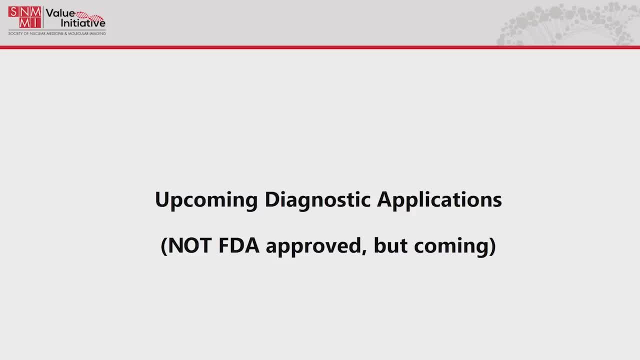 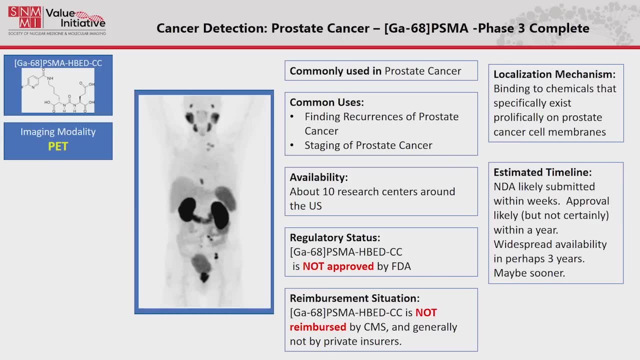 see one is a little bit more diseased than the other. Okay, That's just some basic approved ones. Here's some not FDA approved but coming. This is a very exciting- another exciting prosthetic. This is a prostate cancer agent, gallium-68 PSMA. There's a lot of excitement over this. The choline is good. 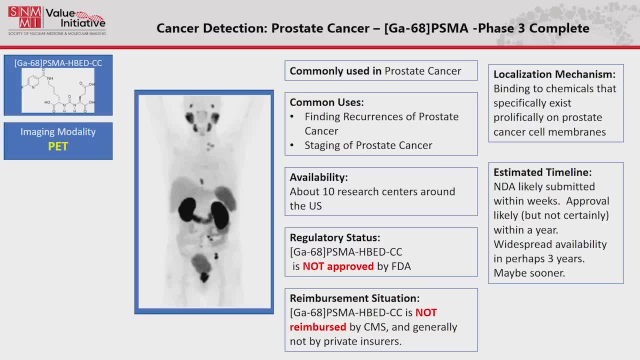 The axiom is good, but the PSMA is seems to be able to detect much smaller lymph nodes sooner. At least that's what the literature is looking like. There is a phase three study that was done, completed between the University of California in San Francisco and UCLA. They are literally a couple weeks away from 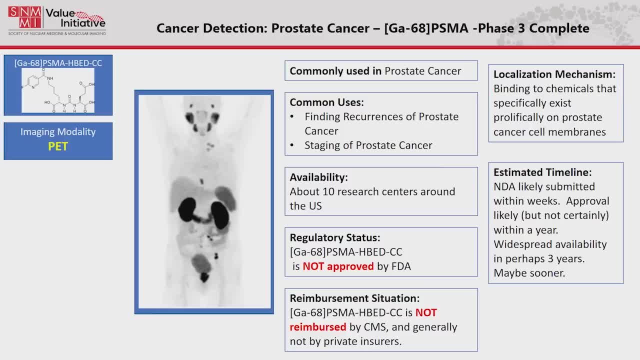 submitting their new drug application. We hope that they get this in Approval. is likely, but not certainly because that's up to FDA within about a year. Widespread availability would be maybe three years or so. That's because not everybody can do it. If we wanted to do it in Iowa we would have to. 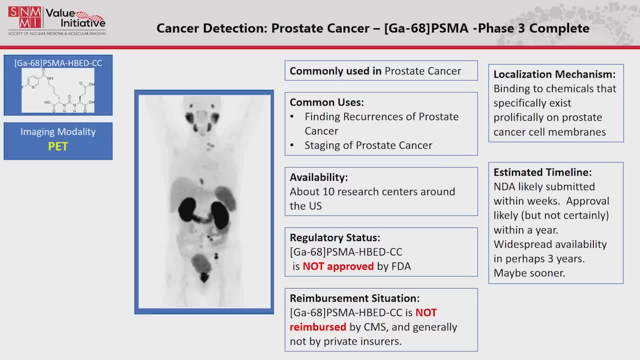 submit an ANDA. That's a whole other application and that goes to the Office of Generic Drugs and takes them about two years to approve those. If it's likely nearby we can go the expanded access IND route, but we'll just have to see on that. 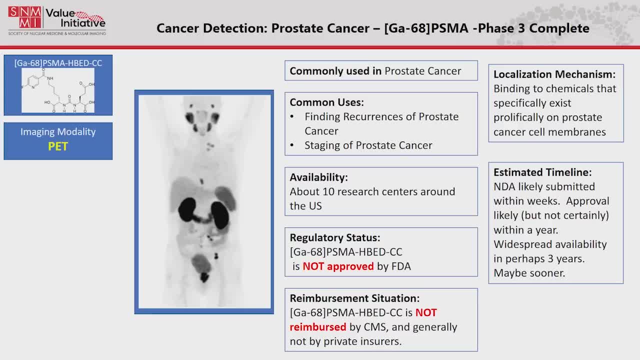 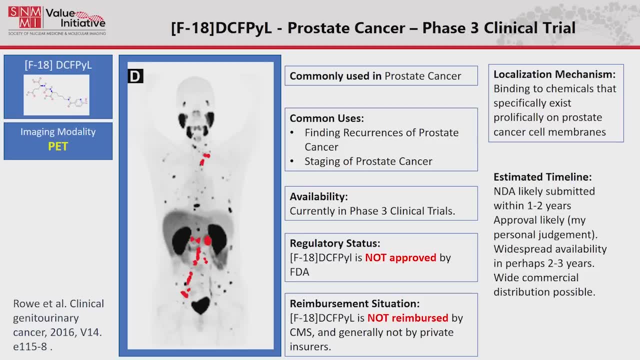 But it's got to get approved first. but it's quite exciting. It's a good agent. Frankly, it's likely a stopgap solution because there is another F18 labeled PSMA, this F18 DCFPYL, which is 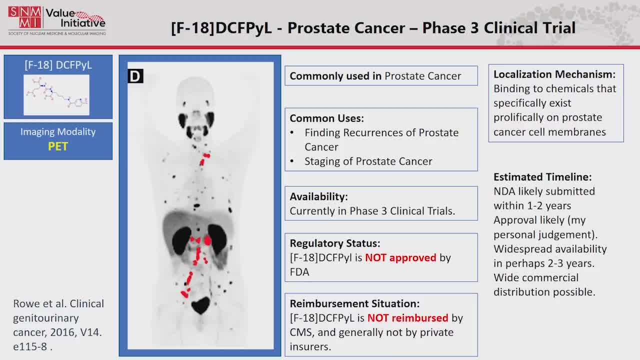 in phase three clinical trials right now. This does pretty much the same thing as the gallium-68 PSMA, but you can make a lot more of it And with the two-hour half-life you can distribute it a lot further. So 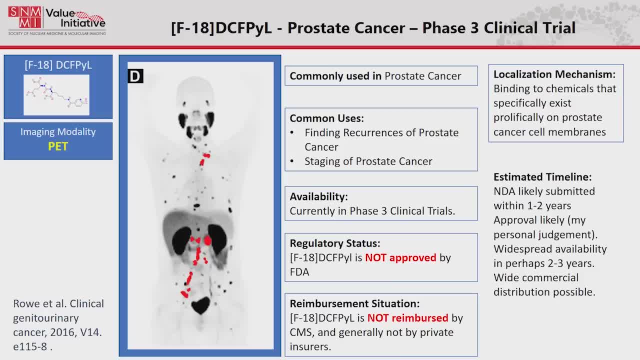 for widespread public availability. this, if I look into my crystal ball, will likely be what most places use two to three years down the road, assuming the phase three clinical trial is successful, assuming they submit the ANDA and assuming FDA accepts it. But that's a very exciting area as well. That first one, the 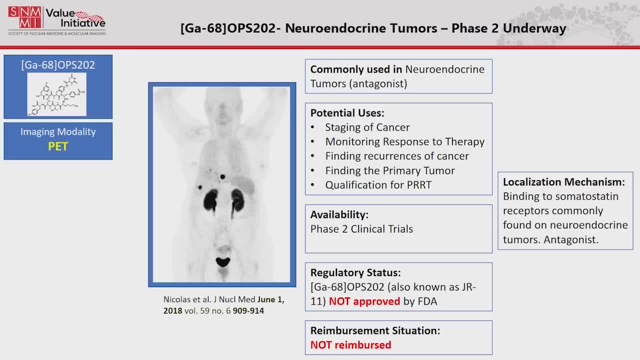 gallium-68 PSMA is not a very good idea. It's a pretty bad idea because it's not really good for the safety of the. The gallium is academically sponsored, The PYL compound is industry And the neuroendocrine space is not static at all. 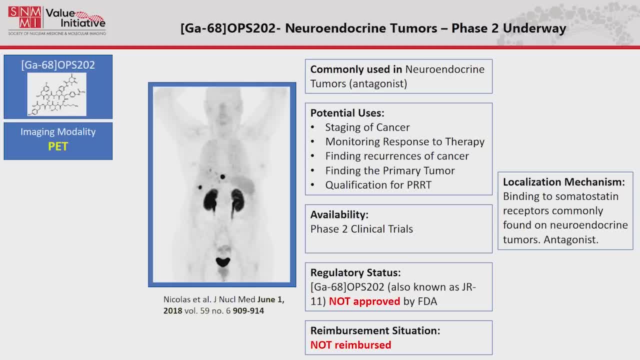 There's this OPS202, which is for neuroendocrine tumors. It works a lot like NetSpot. It works a lot like DOTATOC, except it's an antagonist which, at least it's hypothesized. It has some advantages, both from an imaging and a therapy standpoint. 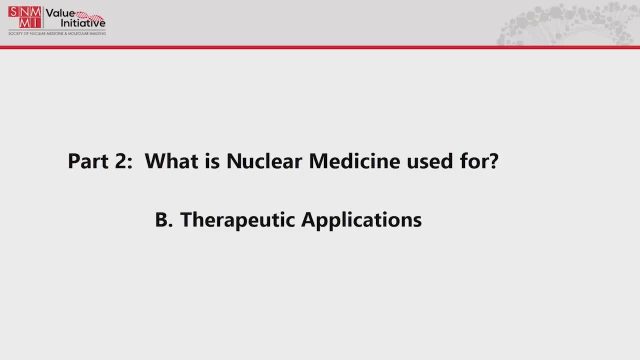 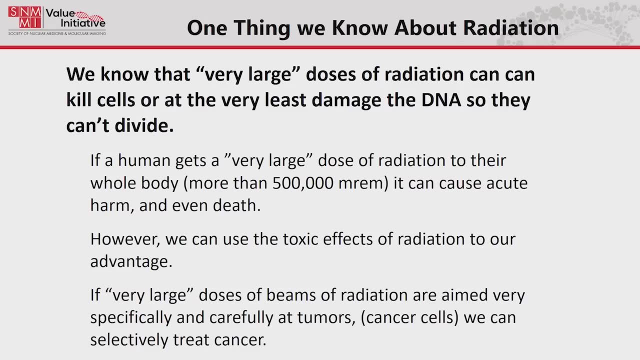 IP2 is not approved yet. It's just phase two And that's really just starting, So it's a better way. I want to move on to therapeutic applications, just for a couple minutes, And to this. we need to begin to understand a little bit about radiation and not just 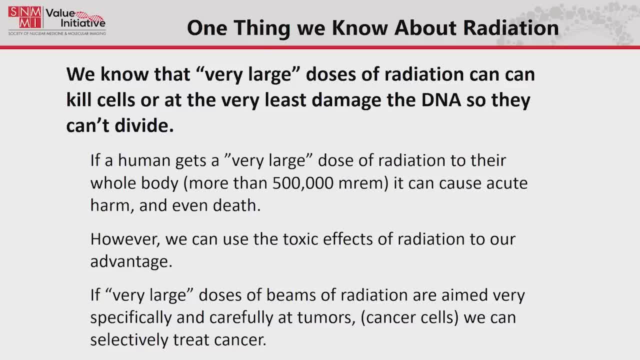 what it can do for us but the harmful effects, And I'm going to get into the doses here in a minute. But we do know that very large doses of radiation can kill cells Or at the very least damage the DNA. so they don't go on. 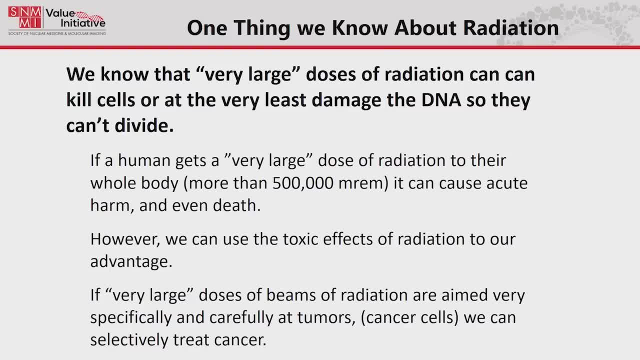 But if a human gets very large doses of radiation all at once- 500,000 millirem- and we'll talk about what a millirem is in a couple of minutes- it can cause acute harm and even death. We know this from Hiroshima and Nagasaki, these kinds of things. that's been studied. 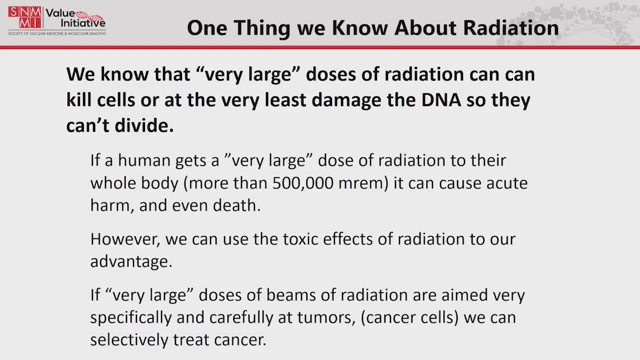 extensively. So we know that radiation is dangerous, particularly in very large doses. However, we can use these toxic effects of radiation to our advantage, Dr John Aucott, PhD. Okay, If very large doses of beams of radiation are aimed very specifically and carefully. 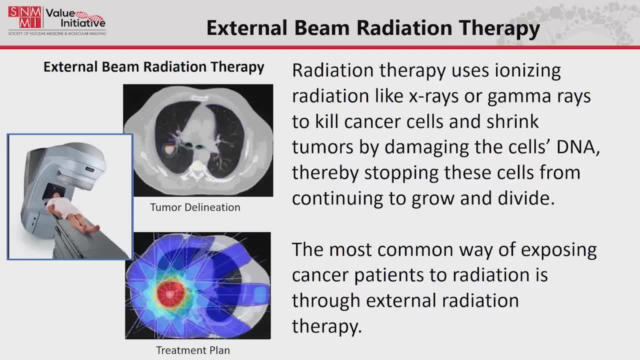 at tumors, the cancer cells. we can selectively treat the cancer. Now, this is not molecular imaging or nuclear imaging. right now I'm just kind of going outside of this to show what external beam radiation therapy does. Here we have a CT scan of somebody going through their lungs and you kind of can see circled. 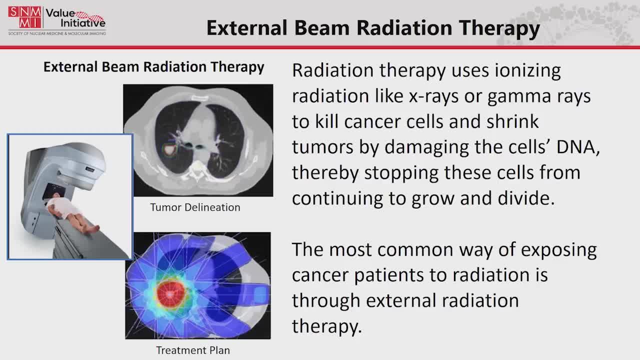 There's a tumor there, And what you do in radiation therapy is you shoot a beam of radiation Which is sublethal from one direction, right, And it goes on through Still a lot of radiation, But then you do it from another angle and then they overlap. 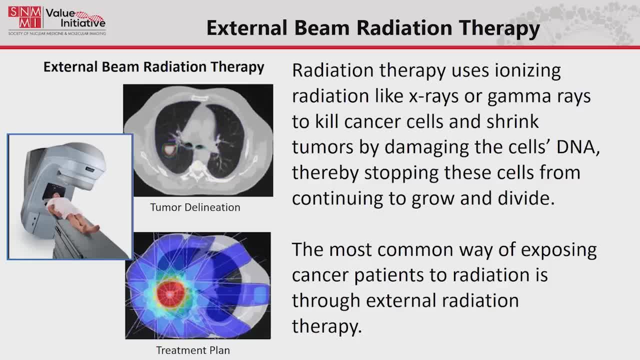 And where they overlap, you now have twice that dose And you do it from another angle, another, And so what you do is you get a lot of dose to the tumor and you get less to the outside, And that's targeting the radiation to the tumor, but not exclusively. 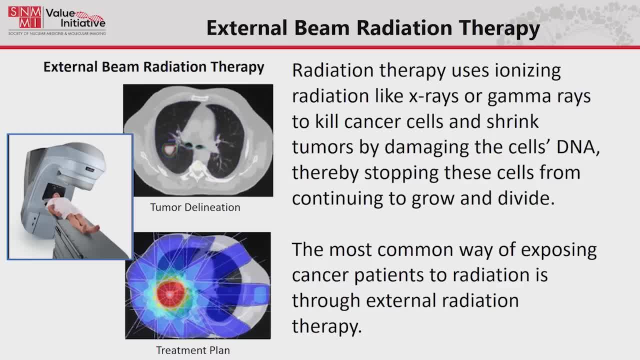 You're still irradiating kind of everything else outside of it. Wouldn't it be nice, Dr John Aucott PhD. Yeah, Dr John Aucott PhD. Yeah. Dr John Aucott PhD. Yeah. 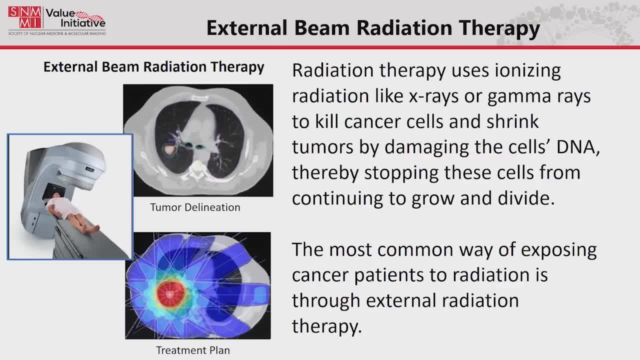 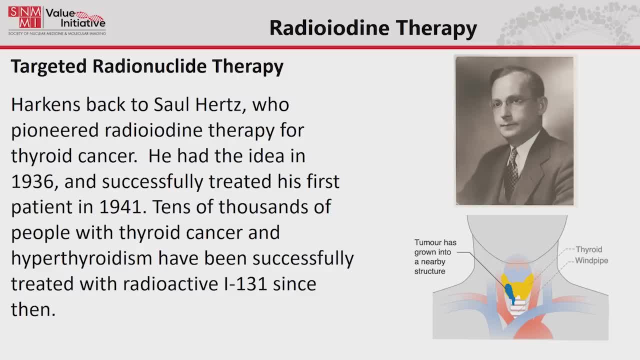 So you're targeting the radiation just to the tumor and not this other stuff. So that's what targeted radionuclide therapy is all about. And those of you who are in PRRT and some of these prostate cancer trials, it all seems. 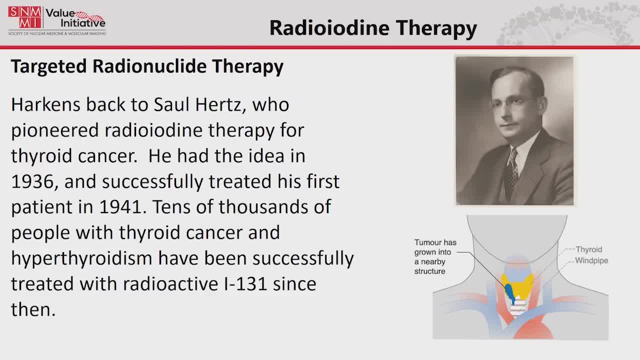 quite new. It's really quite old, In fact. Saul Hertz, back in 1936, had the idea to treat thyroid cancer with radioactive iodine And he treated his first patient in 1941.. You can actually Dr John Aucott PhD. Yeah. 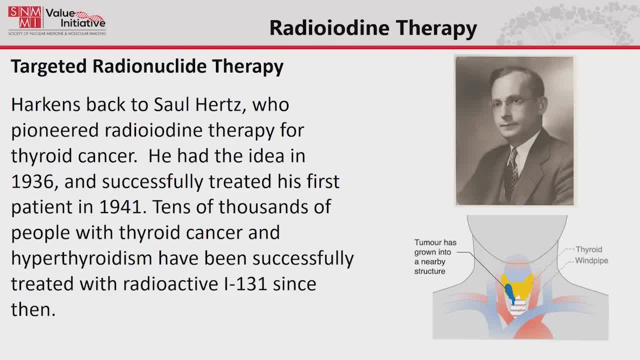 Dr John Aucott, PhD. You can actually ingest it. So we talked about inhaling, We talked about injections. You can actually take a pill that has radioactive iodine-131, goes in the system and the body just moves it to the thyroid and pretty much nowhere else. 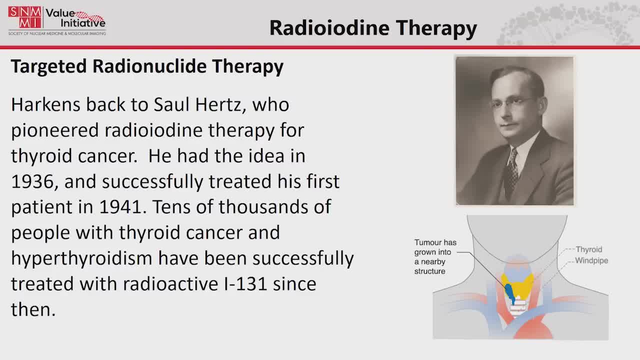 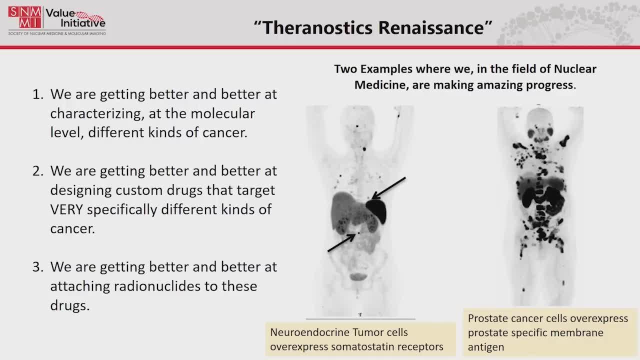 And you can obliterate the thyroid and, more importantly, the thyroid cancer. Tens of thousands of people have been treated with this over the years, So this targeted radionuclide therapy is not new. But what we're getting, Dr John Aucott, PhD, Yeah, 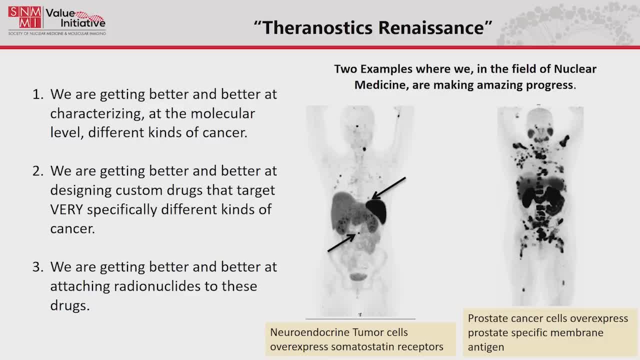 Dr John Aucott, PhD. We're using it a lot more specifically because of three things. One is we're getting better and better at characterizing at a molecular level the different kinds of cancer, the kinds of chemicals that are specifically on the surface of melanoma. 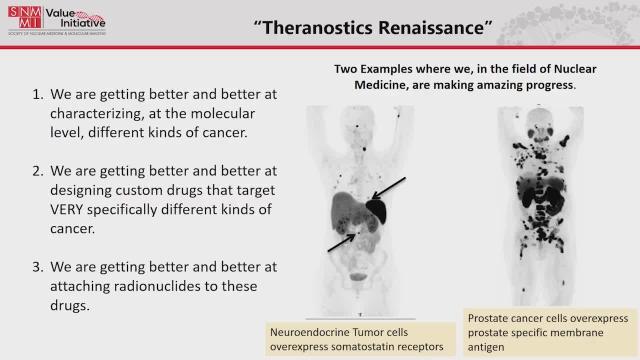 or on the surface of prostate cancer, and we target drugs to this, Then we're getting really good at designing custom drugs that will go specifically to those targets. Then lastly- and sometimes this is the hardest step- then we actually have to take those. 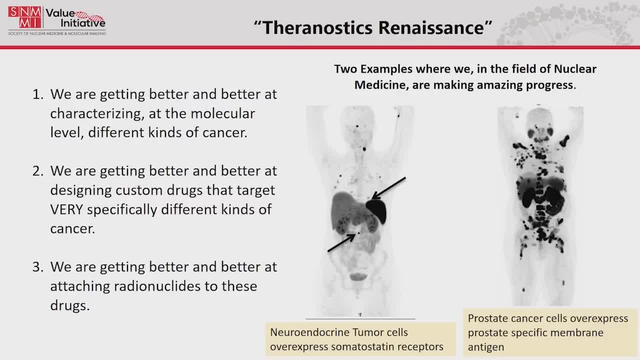 drugs, We have to attach the radioactive atom to it so we can actually get it to, So we can actually follow it. But we're getting very good at these things, and so we're doing it for neuroendocrine tumors, We're doing it for prostate cancer. 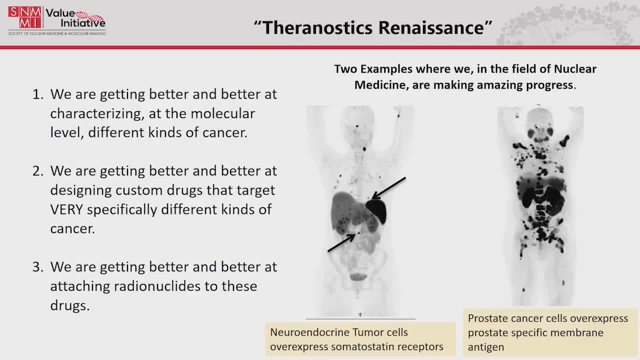 Those are pretty far along, but there are a lot of companies who are developing things for non-small cell lung cancer, for melanoma, for all these cancers, And keep watching this space because it's a very exciting arena, not just for you guys. 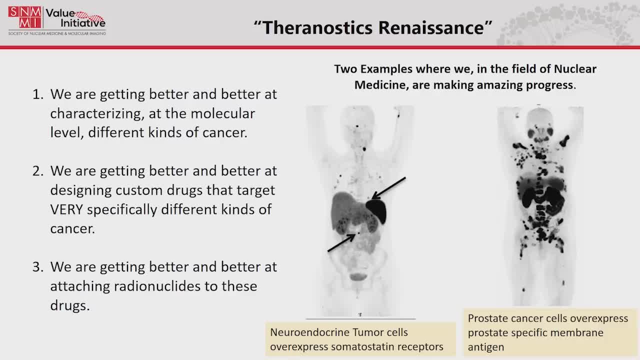 but for companies, because this is a very lucrative thing. And let me go back and just say I mean the good news about these things. it goes really specifically to the tumors. right, You don't have all this kind of crosstalk. 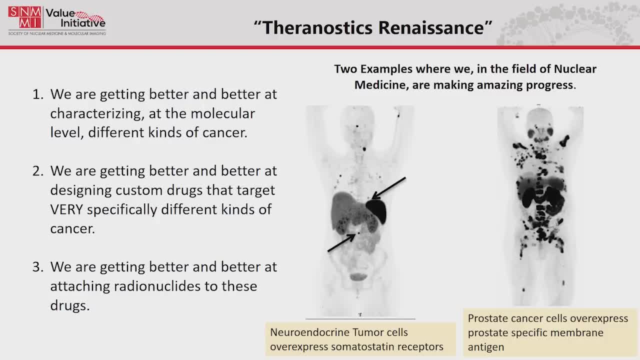 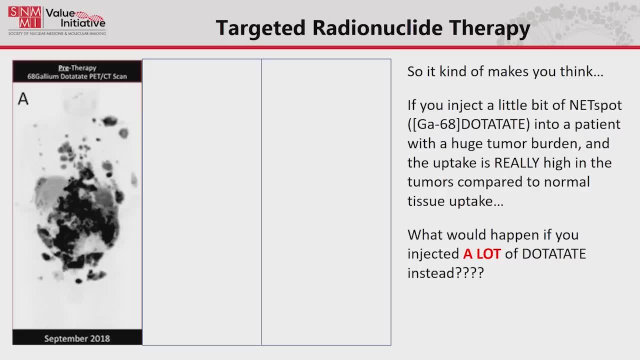 It does go to other organs and all, but not nearly so much. So the more targeted you can be, the better off you are, And so this is just an example. This is with a net spot scan, where somebody has tumor pretty much everywhere. 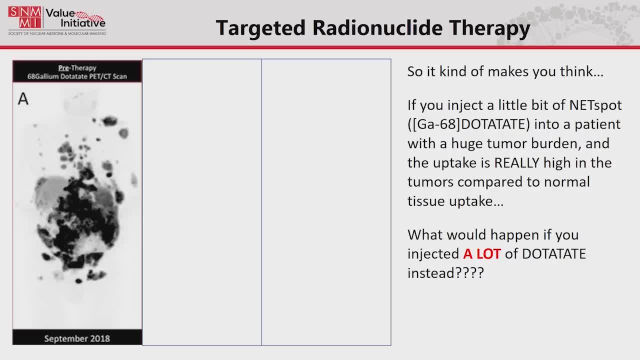 And wouldn't it be nice. And this is just with the gallium right Short half-life. So the idea here is we take that same dotatoc, That's the chemical that binds to the somatostatin receptors. You take that same chem. 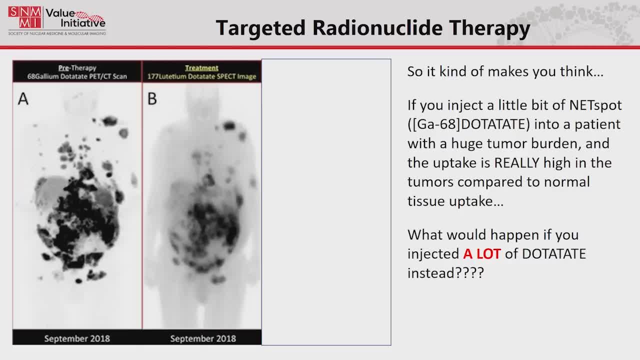 But instead of attaching this gallium-68, you attach lutetium-177.. It has a half-life of about a week, So you inject it into the patient. It goes. Now it gives off a gamma ray so we can image it. 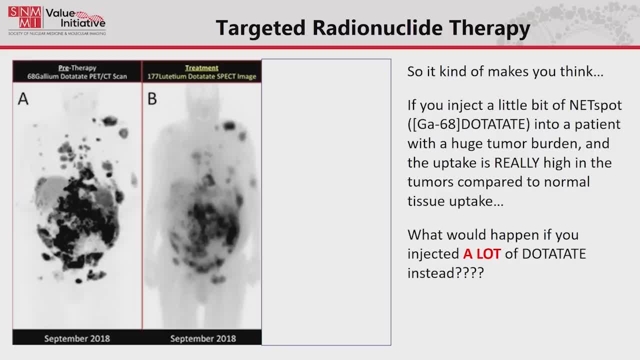 That's why you have an image right. And we didn't just inject a little, We injected a lot, We injected about 100 times more. It's 100 times more And it's got a half-life which is 100 times as long. 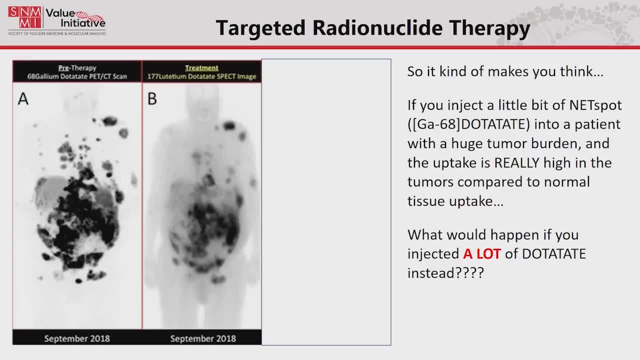 So it's like little machine guns shooting the tumors for weeks until it decays away because it stays bound. And so if you can do that and it happens to be successful, I mean there's no other way to treat this right. And you go through and in some cases- and I could caution you in the literature- they 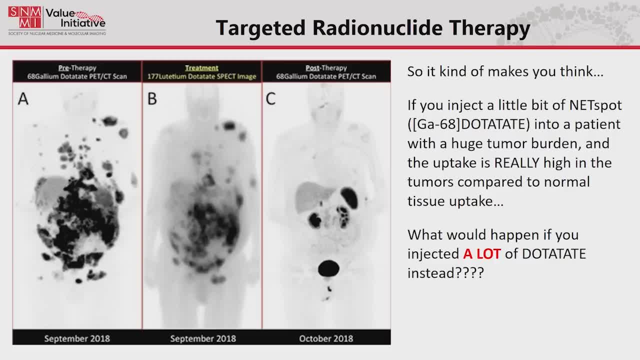 always show you the really good ones, right? So not very often do you have kind of complete responses like this, But it can be. It can be pretty dramatic sometimes, right? And so this is the promise. This is what we're looking for. 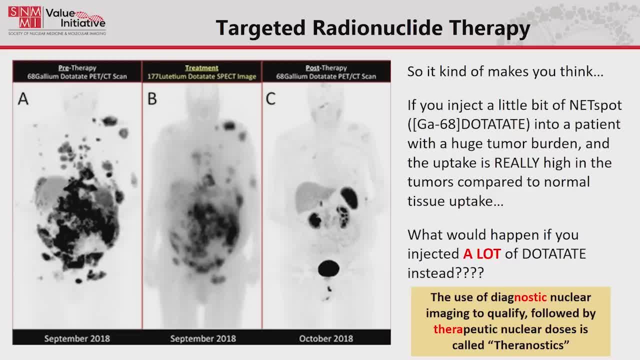 Just so that you know. so the imaging part is the diagnostic, The therapeutic part, the targeted radionuclide, is the therapeutic. And so you might hear the word theranostics. The thera is for the therapy, what we do for the lutetium. 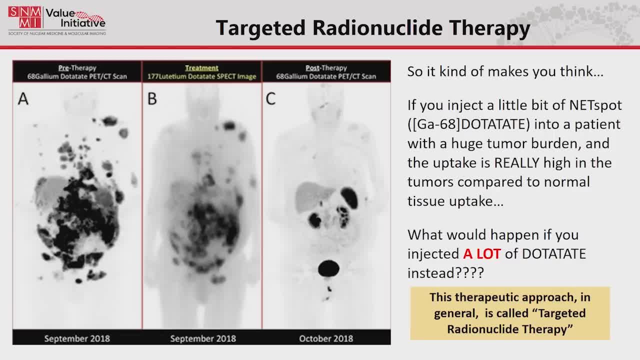 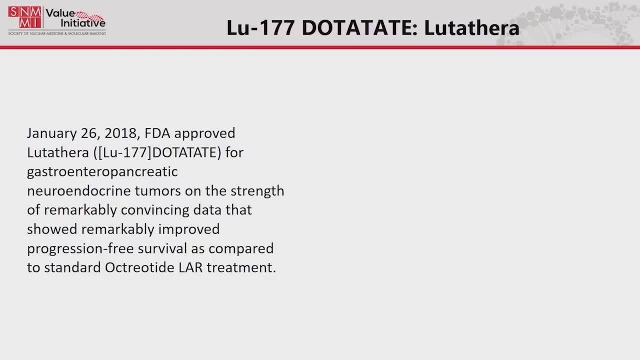 The gnostic is the diagnostic that we do with the gallium in this case- And the therapeutic part is just targeted radionuclide therapy. The good news is We recently have a recent approval lutetium-177-dotatate lutethera. 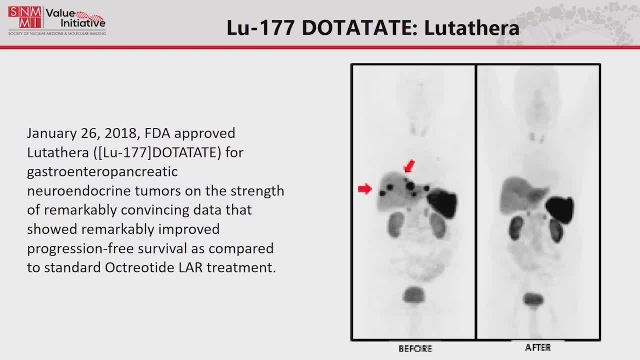 It was approved. Just once again. here's another good example of here's a patient who has a lot of cancer. You treat them and afterwards the cancer largely goes away. This is not necessarily a cure. This reduces the tumor burden and hopefully substantially. 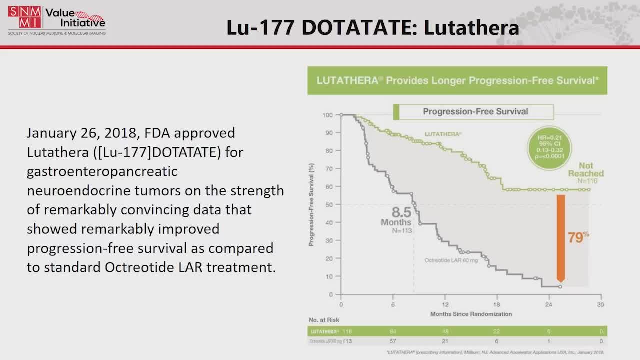 But it can. It's remarkable, and you keep on doing this over time and you can add a lot to it. This is results from the trial. A lot of you have probably seen this. The green line is the people. It's progression-free survival. 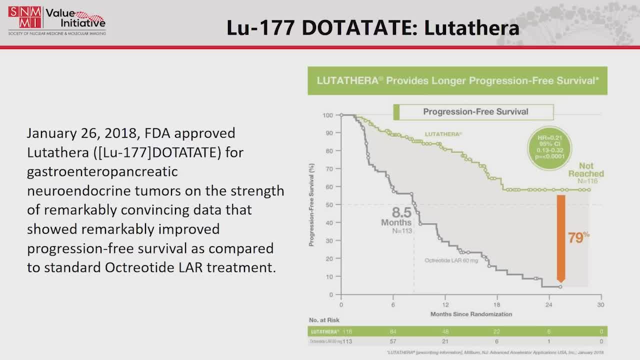 That doesn't mean the cancer goes away. It just means it's not getting any worse right. And so the green line is people who have received the lutethera, and the gray line is people who just kind of had the standard treatment, which is not really much treatment at all. 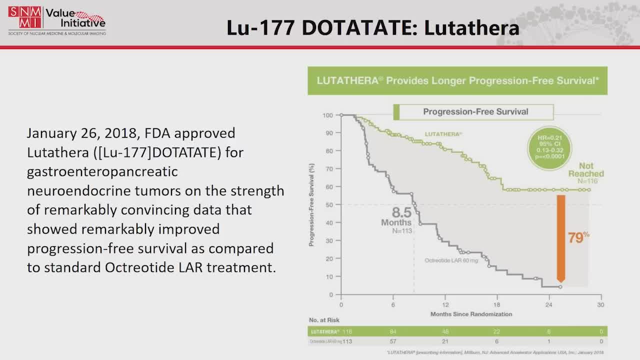 And you can see that. you know, after two years almost all of the minimally treated people had progressed, but about 60% of the people who had been treated, their cancer hadn't gotten any worse and in some cases, gotten better. 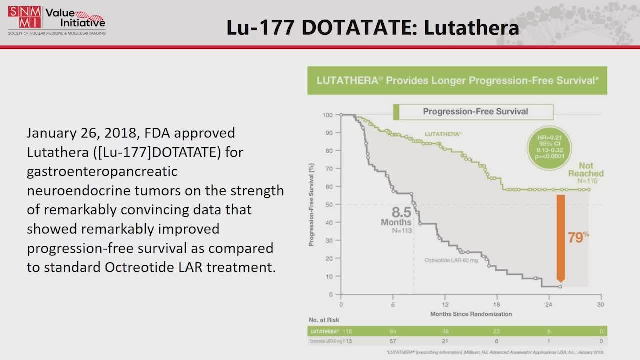 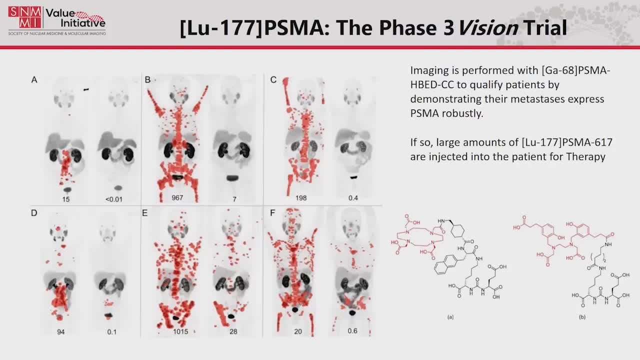 So it's pretty dramatic. You don't usually see plots like this with treatments. If you look at these other chemotherapy drugs, they're not anywhere near as good as this, So this is what's kind of quite exciting. They're doing the same thing with the lutetium PSMA. 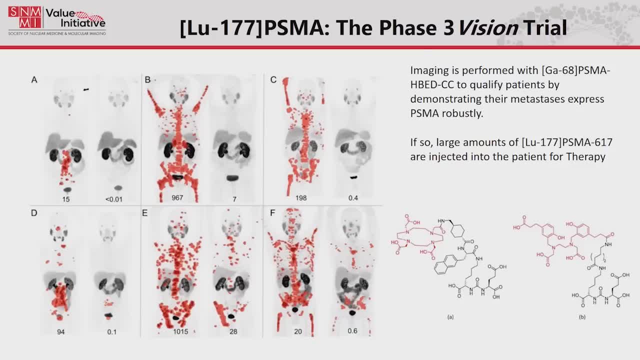 Now this one's in clinical trials, so this is not approved, right? This was the image of the year, I think, last year at the SNMI annual meeting. This was from a group, actually groups down in Australia. These are six different cases. 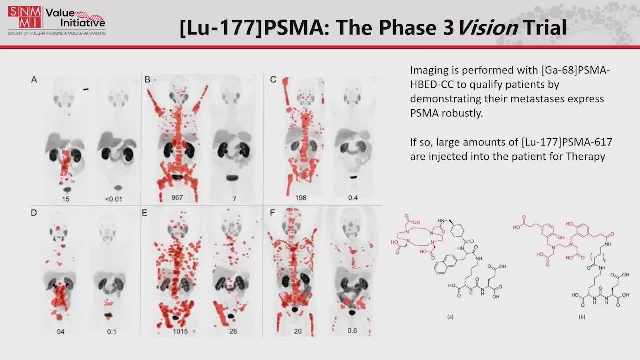 And on the left you can see this: This is from a group. This is from a group. The left-hand side in all cases is the before treatment and on the right is the after treatment. They have artificially kind of shaded where the tumor is in red so you can more easily. 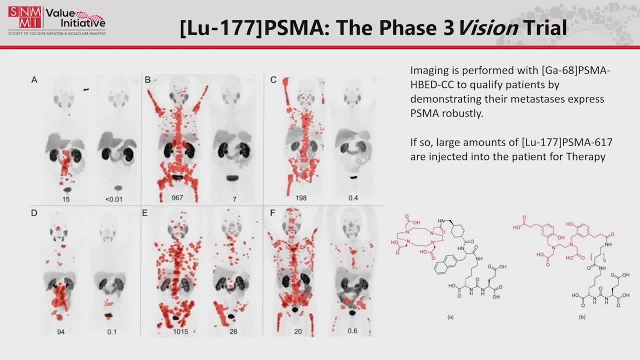 see the before and after: In some cases complete response, In other cases dramatic responses. Once again, this shows great promise. As I said, this is in phase three trials right now and hopefully at least the accrual will be done, probably within about a year. 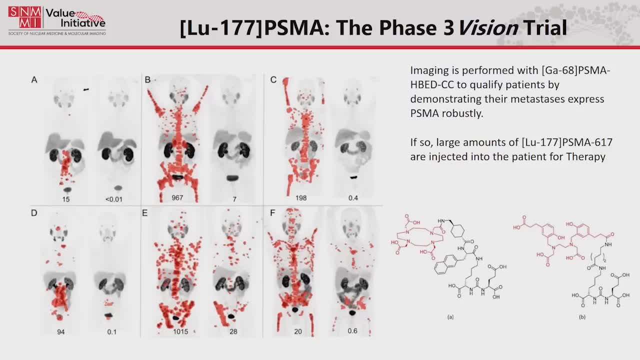 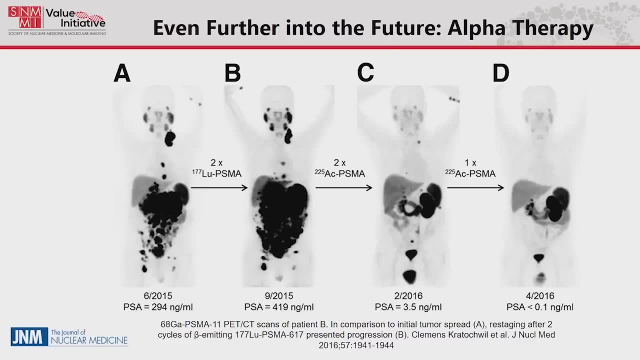 They have follow-up for a couple of years to look at. They look at survival benefit and all, and so hopefully in a few years we'll have some good news on this front, but it's very promising Now. I mentioned alpha particles at the very beginning. you know, shooting bowling balls. 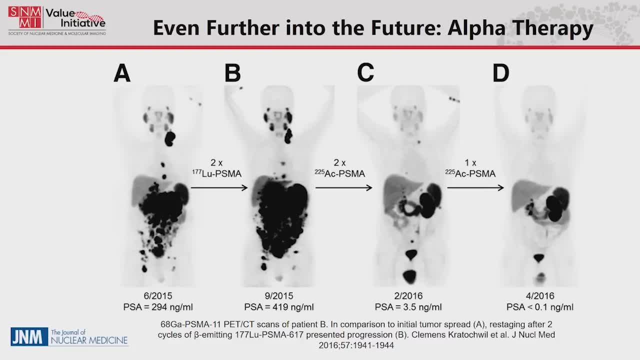 and stuff and also I've been showing these great responses here. This is a PSMA. This is a prostate cancer patient with horrible metastatic disease. They tried the lutetium-177 PSMA. It didn't work And it didn't get any better. 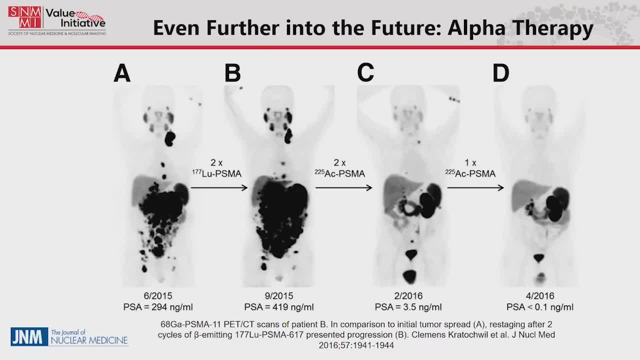 In fact it got worse And if you look at the PSA levels down here, down at the bottom, you can see it actually gets worse. But what they did was they took the same PSMA molecule that targets the surface and they attached actinium-225, which is an alpha emitter. 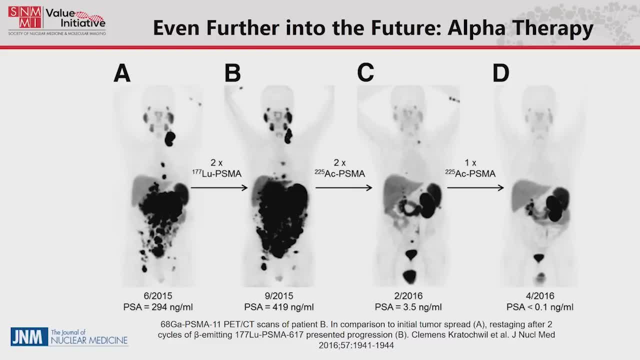 And they gave the patient this two times and they did respond and they responded dramatically. And you can see, after a third, you know, the cancer is almost, you know, almost- completely gone, at least visually, here, Right, So there's a lot of enthusiasm about alphas. 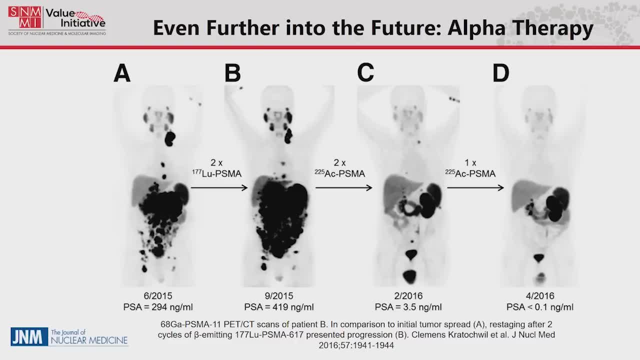 And you've got to be careful about alphas because we don't really fully understand the dosimetry. As I mentioned, you're kind of shooting this bowling ball, so you really have to worry about toxicity issues with this kind of thing And we're really just in the beginning phases. but there's a lot of enthusiasm here. 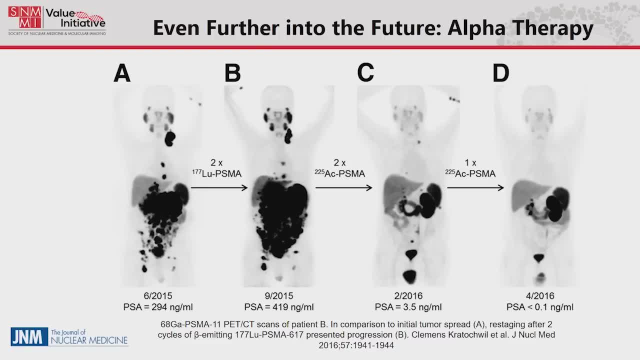 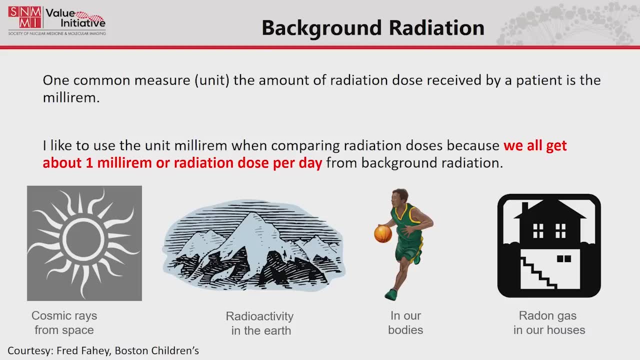 Remember we're years out from doing this clinically, but there's a lot of excitement in this area and a lot of work. Just a few minutes on radiation safety And we are dealing with radiation safety. We are dealing with radioactivity here. 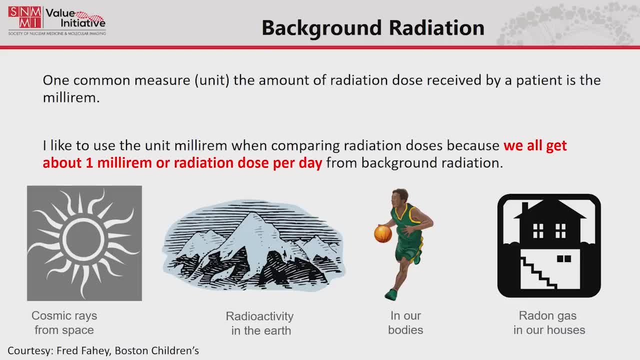 A lot of times in literature you'll see the unit millisievert. For purposes of this talk, I want to use the millirem. It's not the standard unit but I like it because we get about one millirem which is 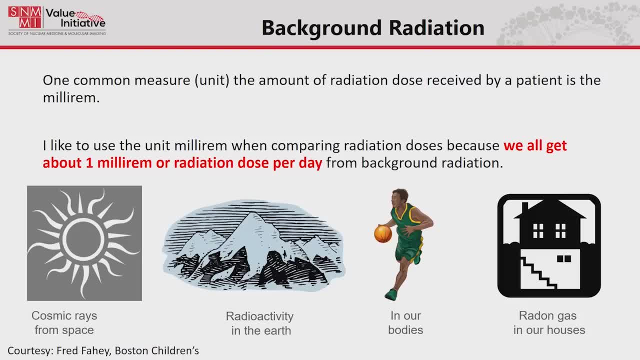 from background radiation. We get about one millirem of radiation dose per day, So that's an easy thing to just kind of remember in the background. So by walking around we got one millirem. Okay, Now where do we get it from? 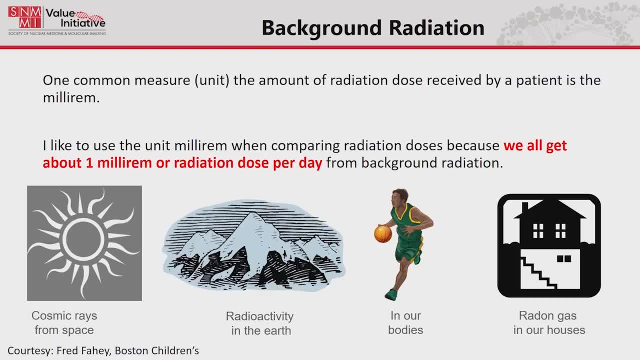 We get it from cosmic rays. We get it from radioactivity of the Earth. There's naturally occurring radioactivity in our body And about half of it we get from radon that we breathe. that's kind of in the basement of our homes, usually about one millirem per day. 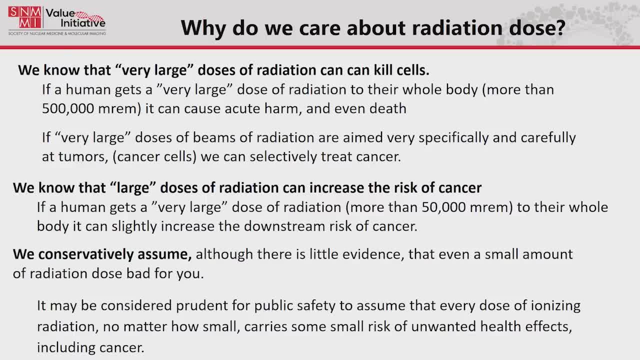 So that's what we all get, just kind of in the background I mentioned before. we get large doses of radiation that can be toxic to us, I will- and kill us, We do know, and that's at the 500,000, so that's 500,000 times we get in a day if you. 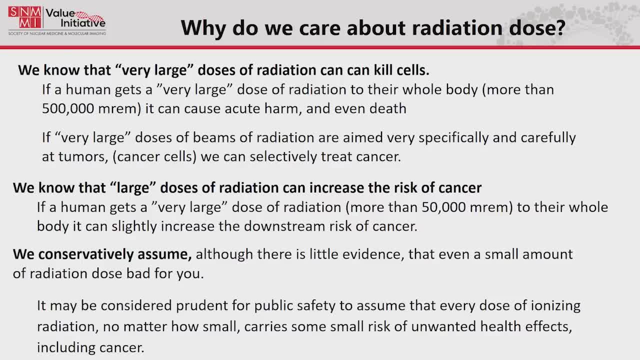 get that all at once, Got about a 50% chance that that's going to kill you. We know that if we go down about a factor of 10 to 50,000 millirems all at once, that's the threshold at which we can start to detect. maybe we get a few more cancers than we otherwise. 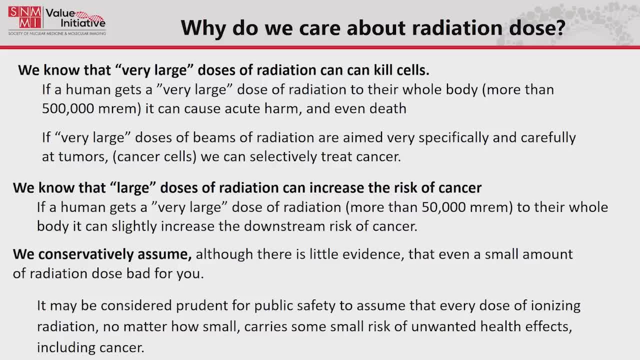 would. Okay, That's where the data actually shows. yeah, we really don't want to go there, So none of the diagnostic tests want to be in a place where we can be there. Most of the tests are way below that And I'll show you some data on that. 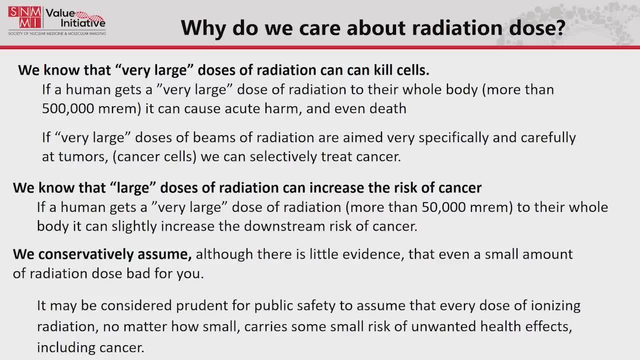 We do conservatively assume- and although there's little evidence- that even a small amount of radiation dose is bad for you. We don't know that a small amount of radiation is bad for you, But we conservatively assume that that is the case. 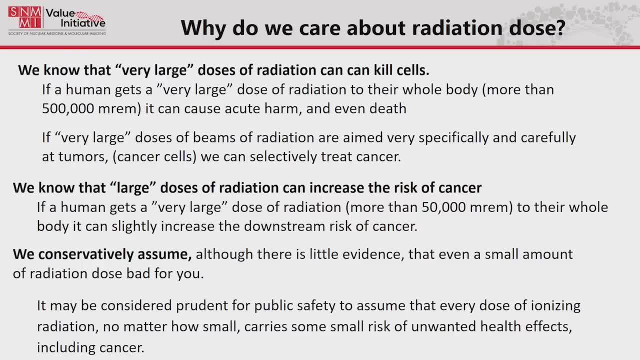 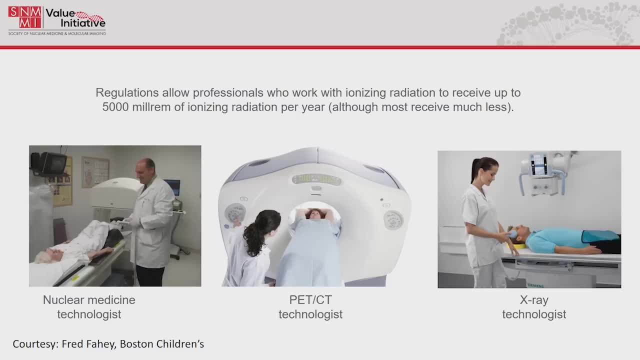 That's all. diagnostic radiology and nuclear medicine is based upon that. So it's prudent for public safety to assume that even small doses of radiation are bad for you, but there's no real good evidence for that, frankly. So. So also benchmark I as a radiation worker I can get 5,000 millirem per year and I'm 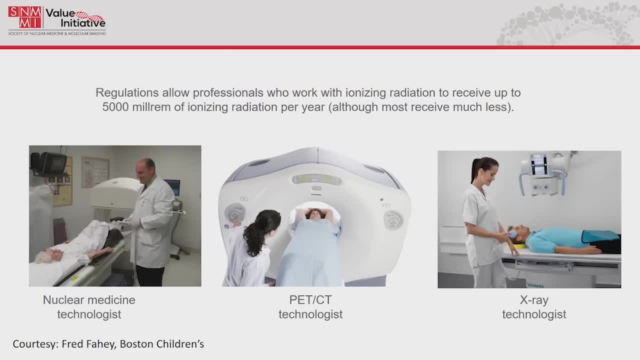 within bounds. That's because we've never noticed, we have never seen any ill effects of radiation at 5,000 millirem per year. So we're in this safety zone okay, And I get. and our technologists who treat, they usually get. they don't get quite up. 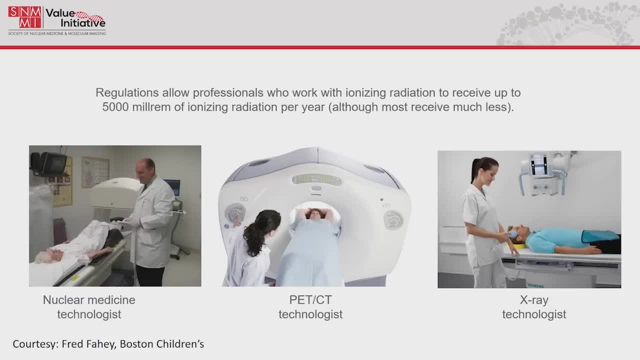 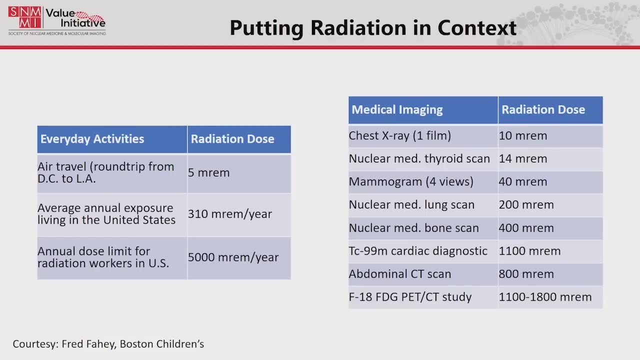 to the limit, but they're on the order of 1,000 or 2,000 annually that they get in administering these patients. They're, they're drugs. So on the left-hand side, everyday dose. Now I flew out here. 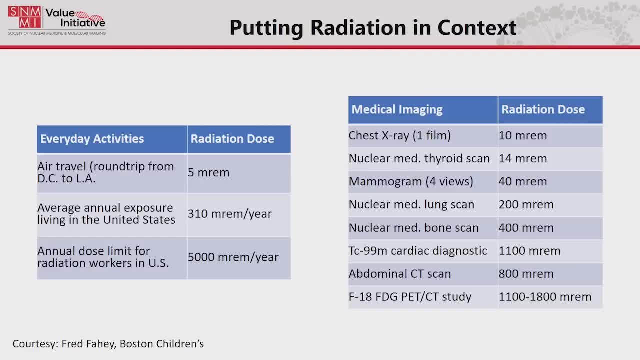 I got 5 millirem because I'm so the the atmosphere does a good job of filtering out cosmic rays. I get about 5 millirem just flying out here from the east coast or the middle, So I get five times background. 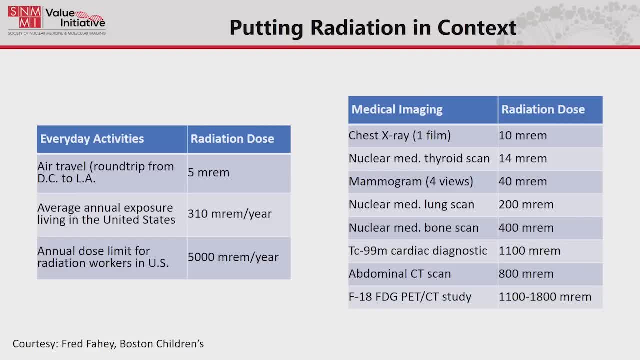 The 310 millirem per year is the average exposure 365 days in a year. that's where I got the about one per day okay, And there's the 5,000 per year Okay. Now, if we look in the right-hand side, we have the standard medical imaging radiation. 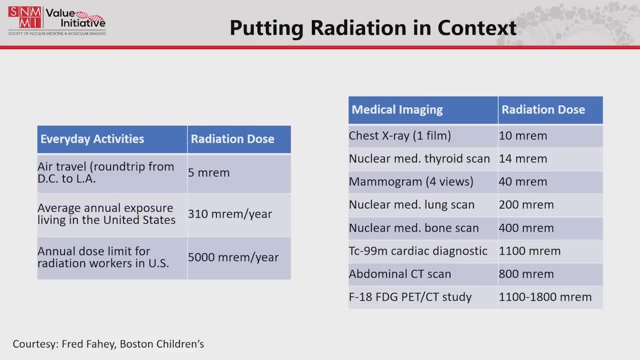 doses. So chest x-ray- do we have pneumonia or not? About 10 millirem is about 10 days of background radiation. Not that big a deal, Remember. a technologist can get on the order of 5,000 per year and not worry about it. 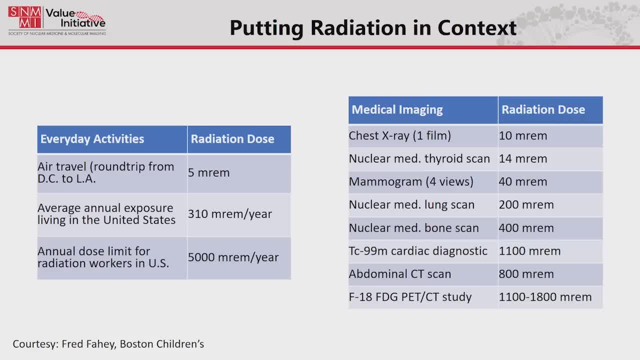 right, If we go down to the nuclear medicine stuff, most of standard nuclear medicine, about two to 400 millirem, that's about a year's worth. you get in in in that And for a PET-CT study you're, you're, you're between 1,000 and 1,000 millirem. So that's about a year's worth. you get in in in that. And for a PET-CT study, you're, you're, you're between 1,000 and 1,000 millirem. So that's about a year's worth. you get in in in that. 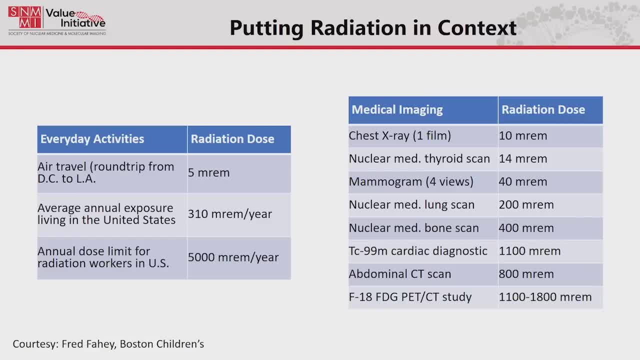 And for a PET-CT study, you're, you're, you're, you're between 1,000 and 1,000, let's say 2,000, which is still below what our technologists get right. And and the bottom line is, for all of these, you're getting it done for a reason, right. 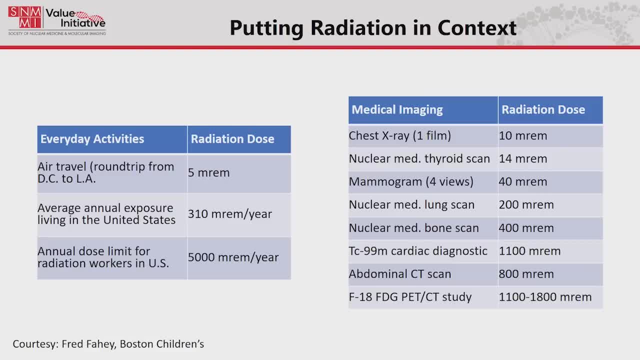 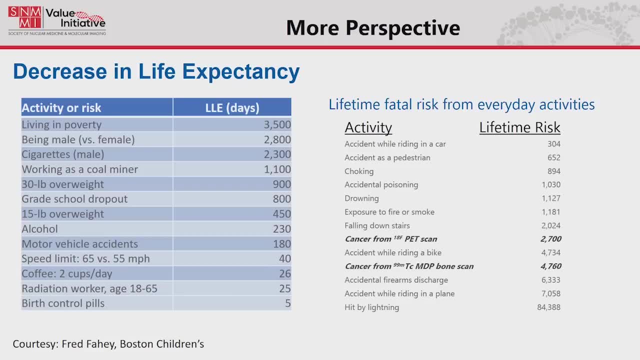 So in the medical imaging biz, this is risk-benefit, risk-benefit And so, and so I don't put a lot of stock in these, but this is for perspective's sake and and hopefully this will be put up on the website and you, you have to, you have to. 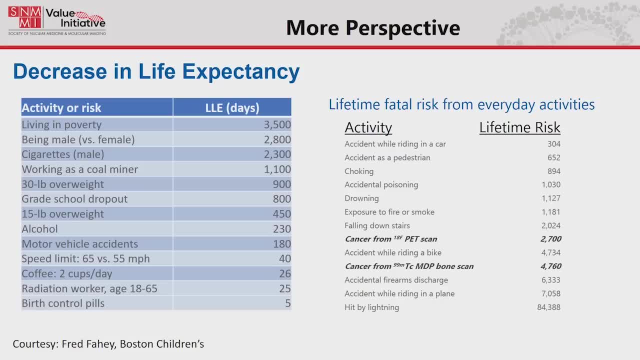 take some of this with a grain of salt. But if you look at at the life expectancy effect of things like living in poverty, you're talking about, you know, 10 years of your life if you do, if you look statistically. 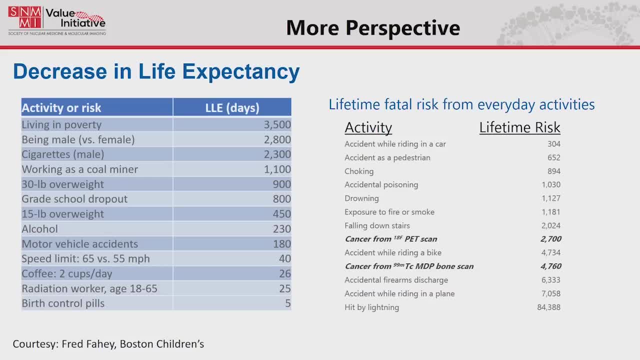 you know. at that, If you're, if you're 30 pounds overweight, you know that's a, that's a, that's a three-year effect. Radiation workers down at that 5,000 millirem statistically. we don't know this, you know. 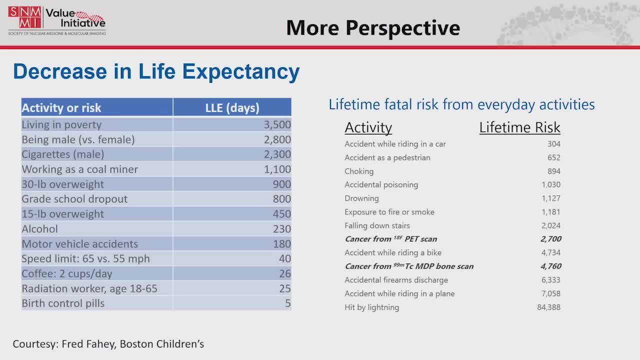 maybe 25 days, but you're getting down. I mean a couple, two cups of coffee, and I'm way more than that. That's, that's what I guess why I need, or you need to worry about, And we have the. we have the lifetime fatal risk from every activity. 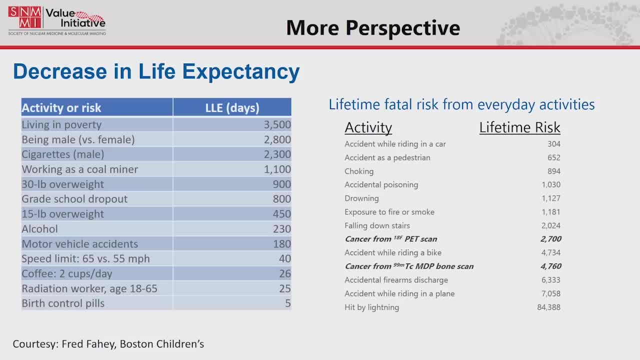 Anyway, these are all. these are all here, and and what they estimate for, like PET scans or bone scans or things like this- these are just worst-case estimates. There's no firm evidence behind it. That's the problem with these things. 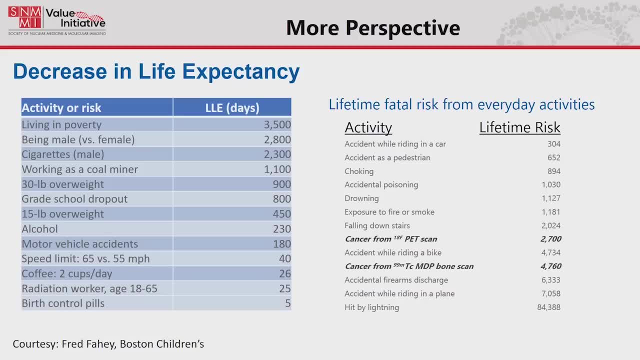 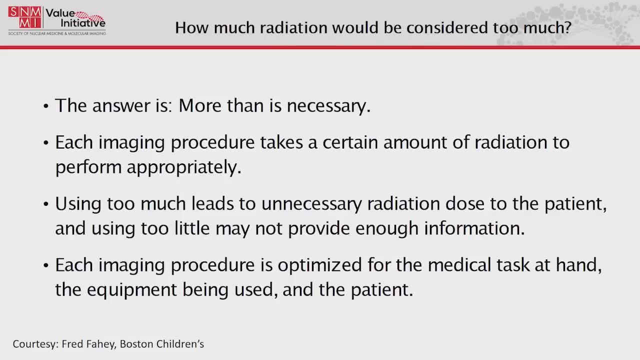 They make it sound like we know, We don't know, We're linearly, linearly kind of projecting backwards from these high doses. So so we, we don't know How much radiation Is too much radiation for a diagnostic test. 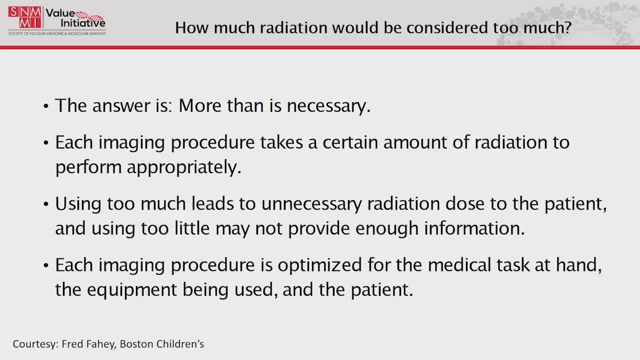 The answer is any more than is necessary right. Each image imaging procedure takes a certain amount of radiation to perform it appropriately. Using too much leads to unnecessary radiation dose to the patient. Too little may not provide enough information. Each imaging procedure is optimized for the medical task at hand. 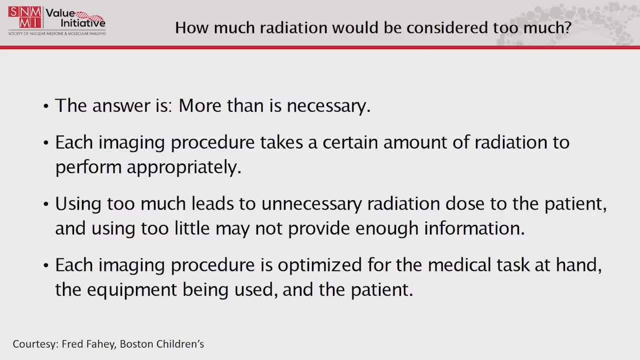 And I'm going to go a little off script here, And so this is my personal opinion, it's nobody else's. When people in particular get PET scans, They look at the patient, They look at the patient, They look at the study. 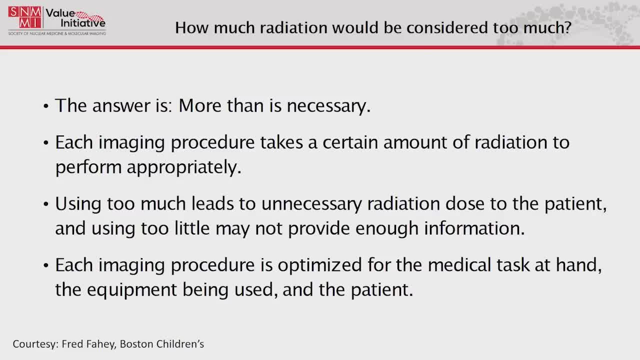 They look at the physical side of it. So you really want the test, you know the test to be done right. So when you take a picture with your cell phone and it's kind of dark and all you can go into Photoshop and you can try and 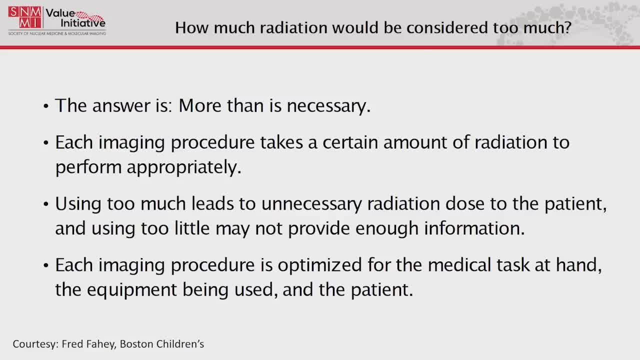 but if the information isn't there, the information isn't there. So you need the right exposure And we work very hard to do that. but as far as I'm concerned, it's all about the image quality right And because you have, in general, life-threatening disease. 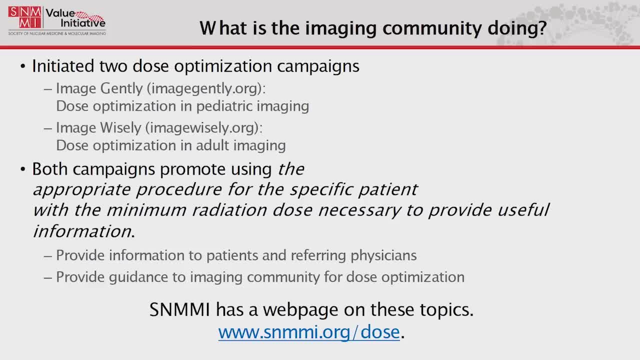 you want to make sure you get it right. What is the image community doing? There's an Image Gently campaign for pediatric imaging. There's Image Wisely for dose optimization for adult imaging. The society takes this very seriously. We're tweaking.